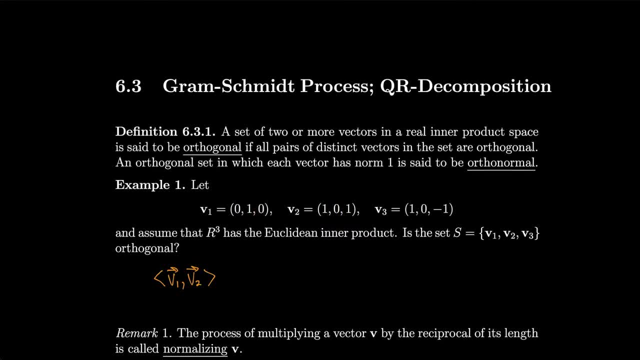 zero, and then the zero cancels out this one. So that should be zero. But notice, if you take v1 and dot it with v3, you'll also get zero. And if you take v2 and dot it with v3, you'll also get. 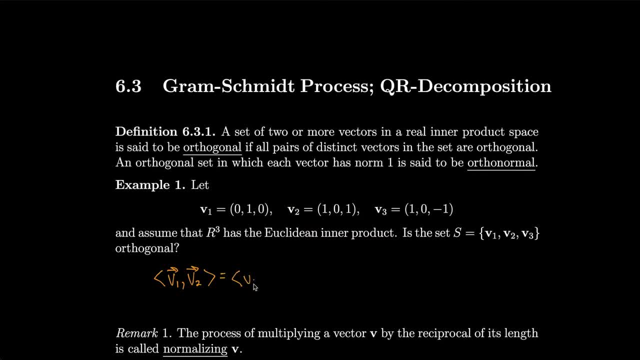 zero. So all of these dot products, which are the Euclidean inner products, are all equal to each other and they all equal zero. So that implies that, yes, sa is Orthogonal. The process of multiplying a vector v by the bar reciprocal of its length is: 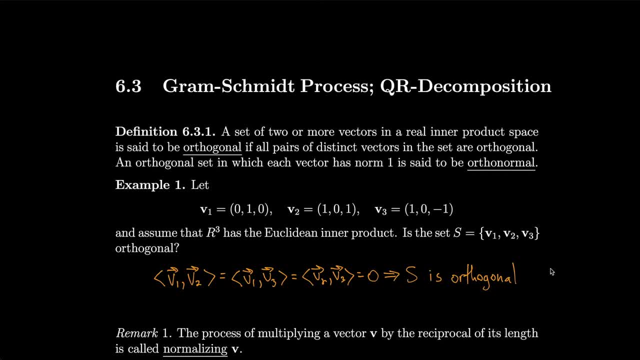 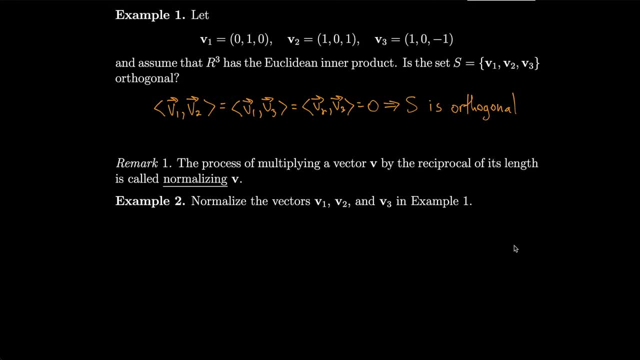 called normalizing v. So as an example of that, how about we normalize the vectors from example one? So let's get the length of v1.. and notice, we just have one there. So when we take 1 squared, take the square root, we'll just get 1, according to the Euclidean norm. 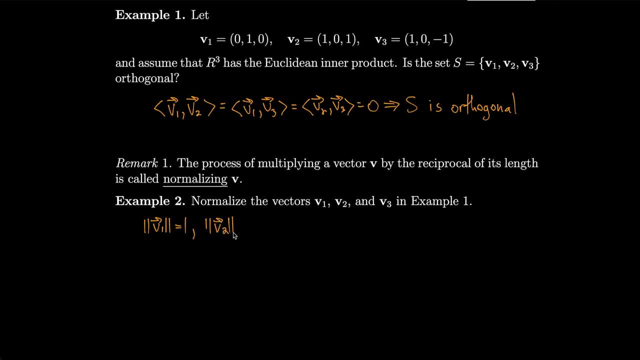 And we'll get the length of v2.. And that's going to be the square root of 1 squared plus 1 squared, so a square root of 2.. And then we can get that the length of v3 is square root of 2 also. 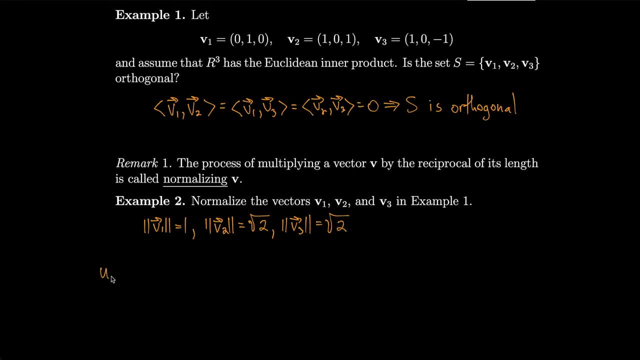 So that means that we can get u1 equal to v1 divided by its length, and that'll be the normalization of v1.. So if we divide v1 by 1, then we just get v1, so 0, 1, 0. 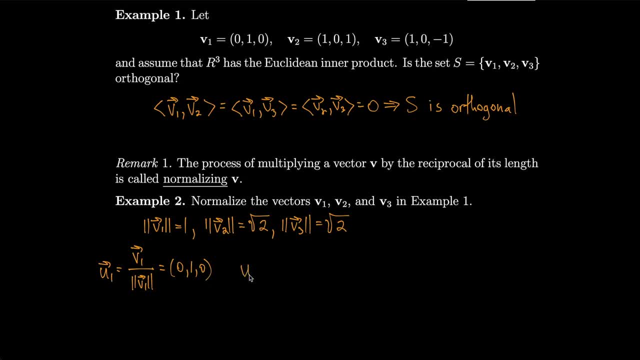 So v1 is equal to its normalization, But for u2, that's v2 divided by its length. So that's 1 divided by square root of 2, 0, and 1 divided by square root of 2.. 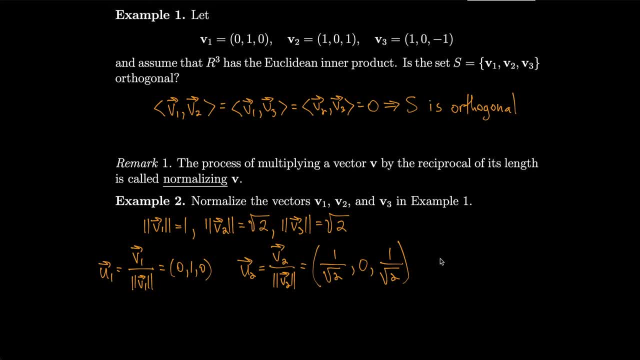 So u2 is not equal to v2.. Let's get u3 now, So that'll be v3 divided by its length, And that's equal to 1 over root 2, 0.. Minus 1 over root 2.. 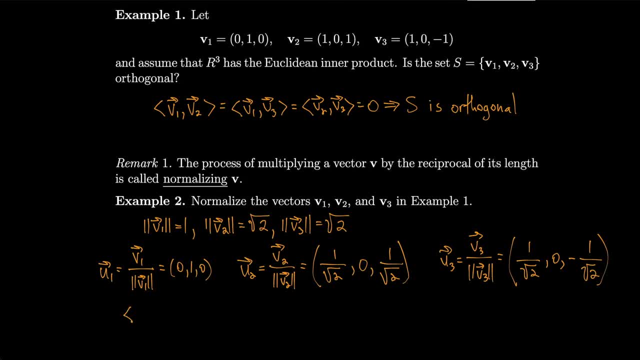 Now let's take the inner products, just as a check. Let's take u1, inner product with u2.. Notice, we still have the 1 in the middle and 0s otherwise. So when we multiply the corresponding components, this 0 kills that 1, and it'll just be 0. 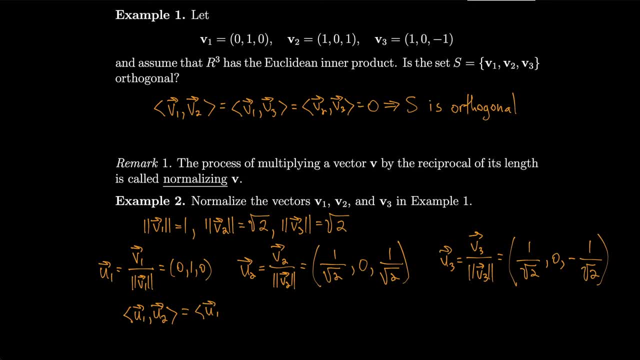 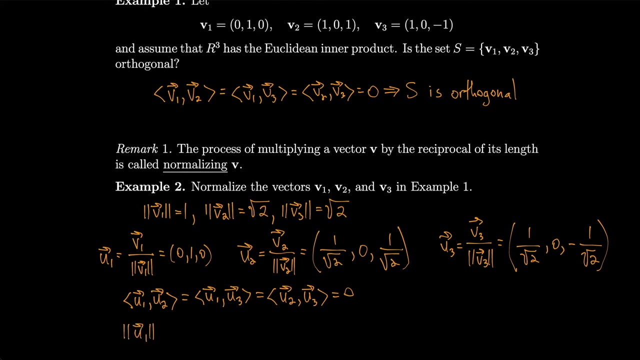 So same thing for u1.. u1- inner product with u3, that dot product is also 0, and u2, and u3. So those are all 0. But when we looked at the lengths u1,, u2, and u3,, 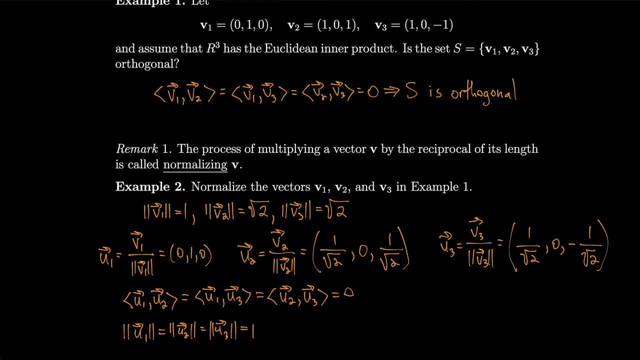 would all have to have length 1, right? If you take, Well, obviously this is length 1.. But if you take this quantity square it, add it to this quantity, you get half plus half is 1.. And for the last one also, half plus half is 1.. 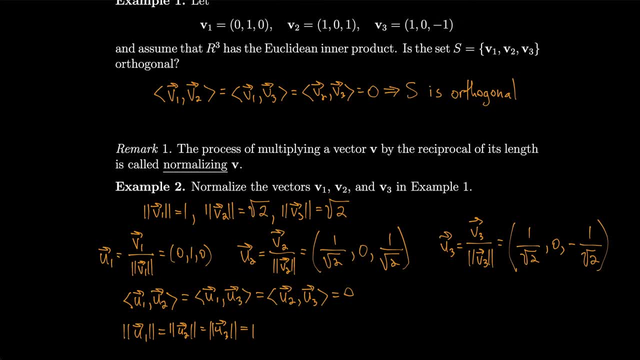 So all of the lengths of our normalized vectors are 1.. That's no coincidence. Dividing by its length will produce a vector with length 1.. So that means that we have vectors that are orthogonal and have length 1. So we now have an orthonormal set S. 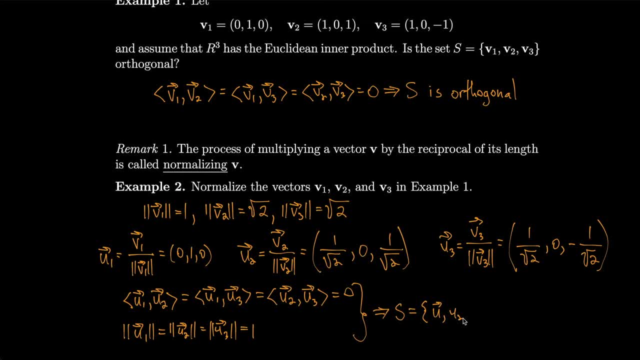 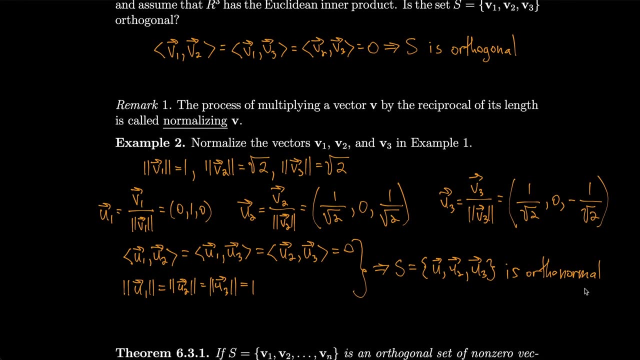 So S equals u1,, u2, and u3 is orthonormal, Whereas the set of Vs was just orthogonal. So to get an orthonormal set we just need to find an orthogonal set and divide so that the vectors are normalized. 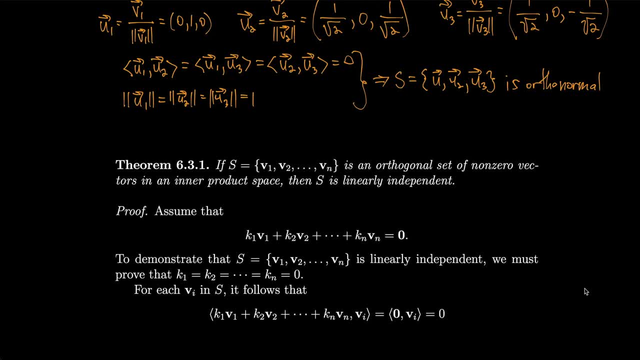 If S equals V1 through Vn is an orthogonal set of non-zero vectors in an inner product space, then S is linearly independent. To prove this, let's assume that K1, V1 plus K2, V2 and so on, through Kn, Vn is equal to zero. 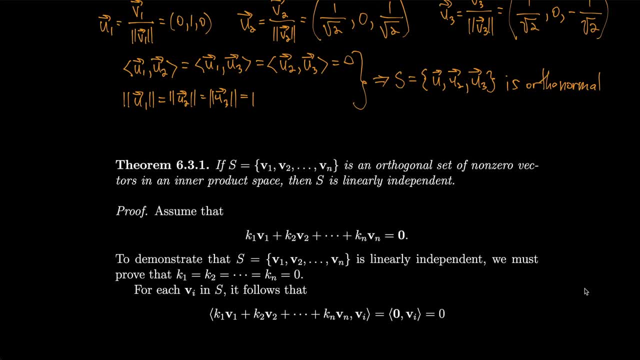 So we have to demonstrate linear independence, We have to prove that all of the constants are zero. So for each Vi and S it follows that K1, V1 plus K2, V2 and so on, If we take that inner product with V1,. 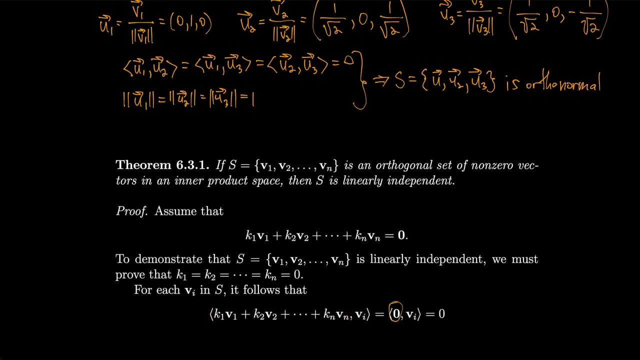 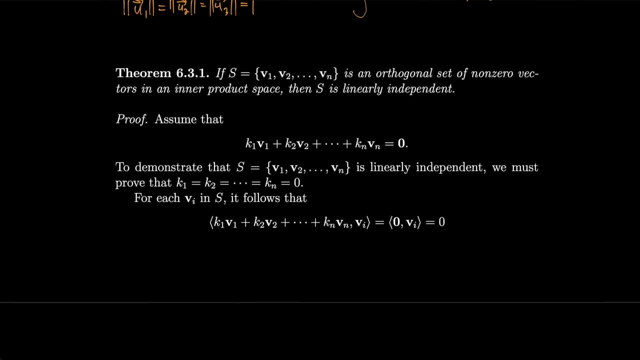 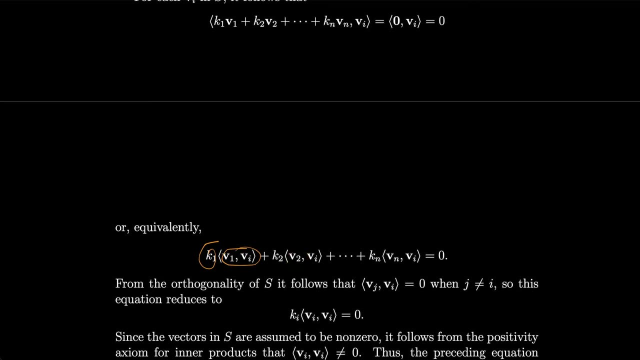 then that's the inner product of zero with Vi, Then that's the inner product of zero with Vi. So that's just zero. So that's the same thing as saying that the constant times, each of those terms, gets you to zero, right. 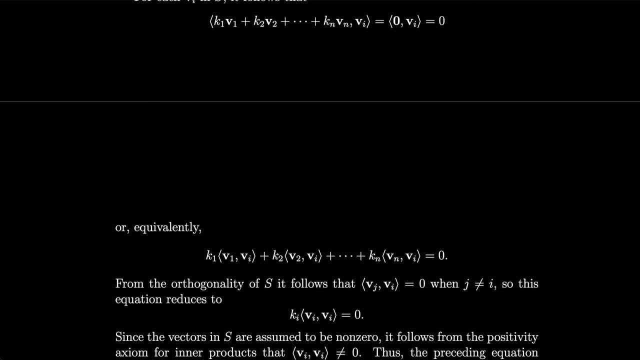 Because we could pull the constant out of the inner product by the properties of inner product and then separate them out into each of their own inner products with Vi. So from the orthogonality of S it follows that the inner product between Vj and Vi must be zero whenever j is not equal to i. 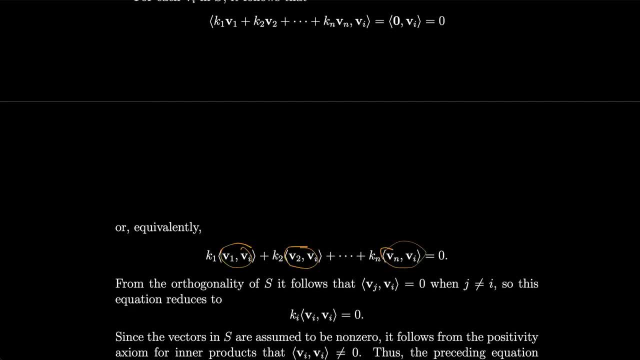 We have to have all of these guys equal to zero. whenever we have that. the V subscript is not the same as this V subscript, So that's the same thing as saying that Kivii is equal to zero, Since the vectors in S are assumed to be non-zero. 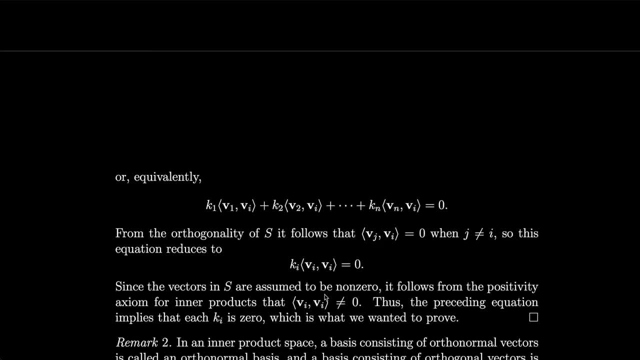 it follows, in the positivity axiom for inner products that we have, that the inner product of V with itself is not equal to zero, because V is not zero. So that means that the Ki has to be zero, which is exactly what we wanted to prove. 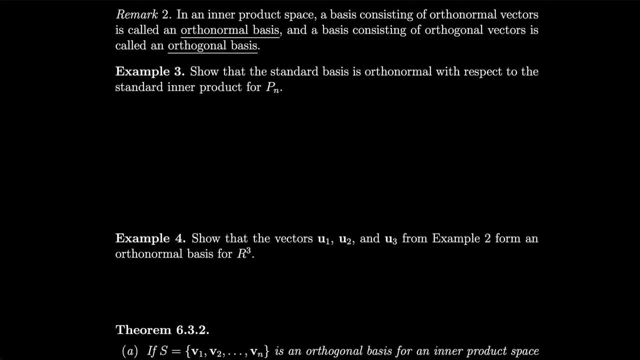 In an inner product space. a basis consisting of orthonormal vectors is called an orthonormal basis. A basis consisting of just orthogonal vectors is called an orthogonal basis. Let's show that the standard basis is orthonormal with respect to the standard inner product for Pn. 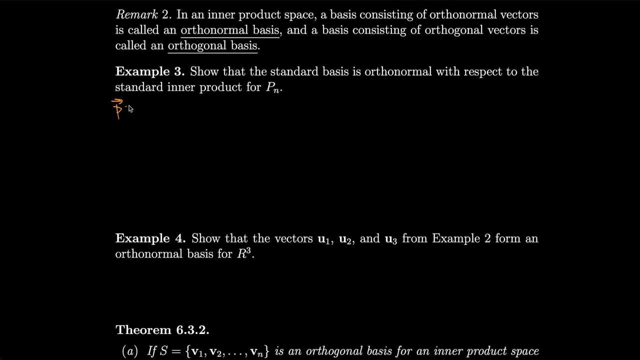 So I'll write out some polynomials. How about I write: P equals a0 plus a1x plus well, so on, through a and xn. and I'll get another vector in Pn by writing another polynomial: Q equal to b0 plus b1x, and so on. 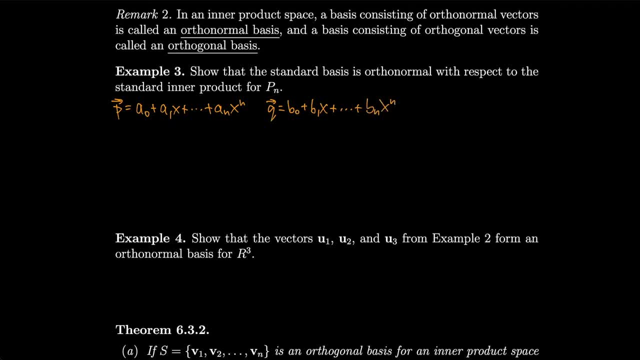 Through bn, xn. So now let's take the inner product of P with Q. So that means that I just multiply the coefficients, So a0, b0 plus a1, b1 and so on, all through an bn, And I'll take the length of P. 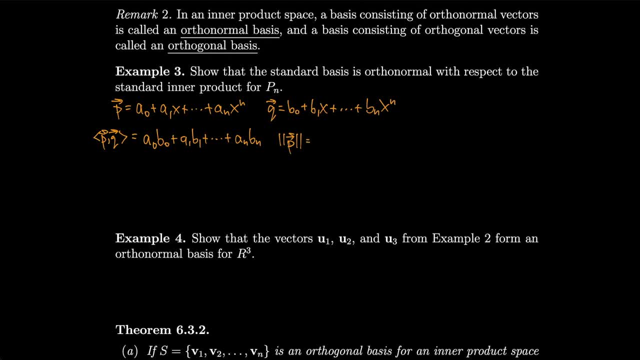 That's the square root of the inner product of P with P. So that's just the square root of all of those coefficients squared, So a0 squared plus a1 squared and so on, through an squared. And that means that I would like to look at the 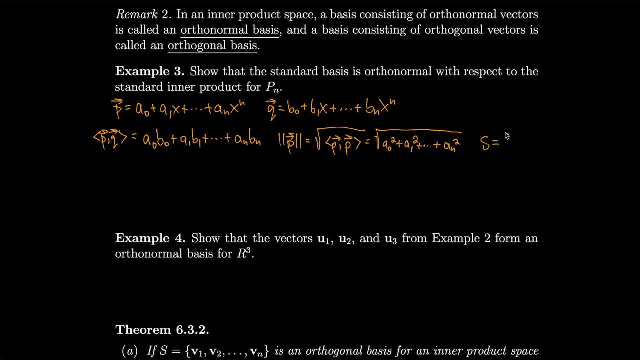 standard basis. Let's see: s equals 1x x squared through xn. So I need to show that this is orthonormal. I have this as the inner product. I have this as the way to take the length. So let's use those facts and check s. 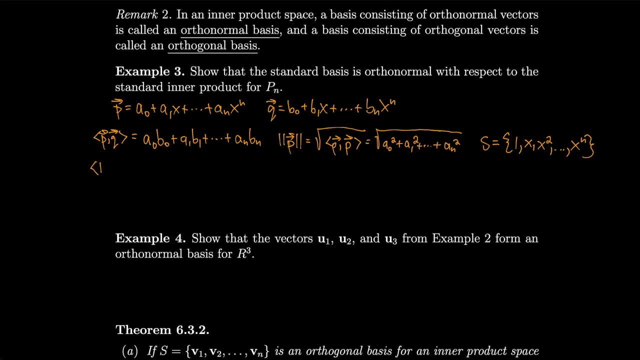 So how about I take the inner product of the first one, 1 with x? Well, the inner product of 1 with x would have the coefficient 1 times the coefficient in this polynomial x. But this is: you could rewrite 1 as like 1 plus 0x and you can write x as 0 plus 1x. 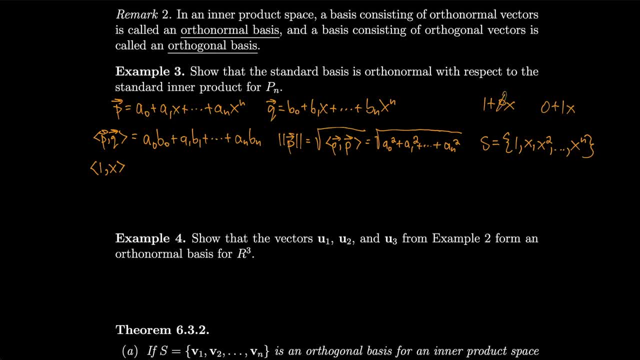 Notice, when you take 1 times 0 and add it to 0 times 1. You'll just get 0. So the inner product of 1 with x will give you 0. And similarly, because you only have one coefficient in each of these vectors in this set. 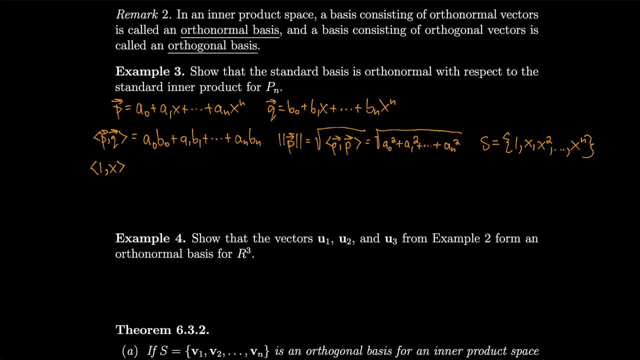 and the coefficients don't match up. they're all in different places. All of the rest of the coefficients in each of these is 0. Whenever you multiply them out, you're going to get 0. So inner product of 1 with x will give you 0. 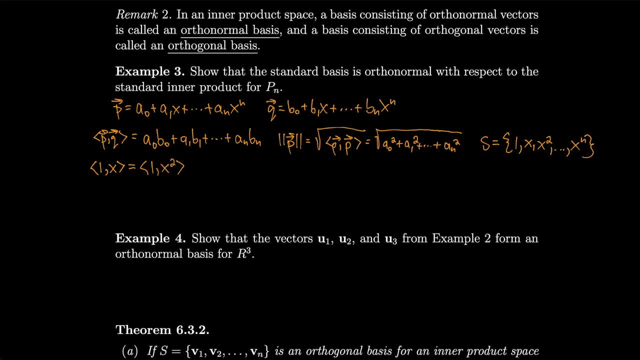 The inner product Of 1 with x squared would also give you 0, and so on. So the and then, if you go to the inner products of x with each of the successive vectors, x with x squared will give you 0.. X with x cubed will give you 0, all by the same reasoning, and so on. 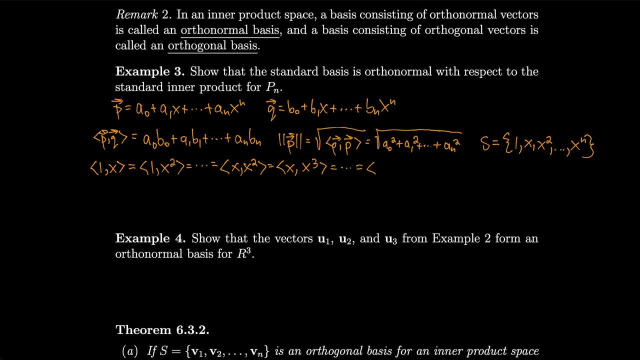 So you could take, keep taking inner products all the way through all the powers, x and minus 1, all the way up to x, n, and they'll all be 0.. Let's get the lengths Now, the length of 1.. Well, clearly, the square root of 1 squared will just be 1.. 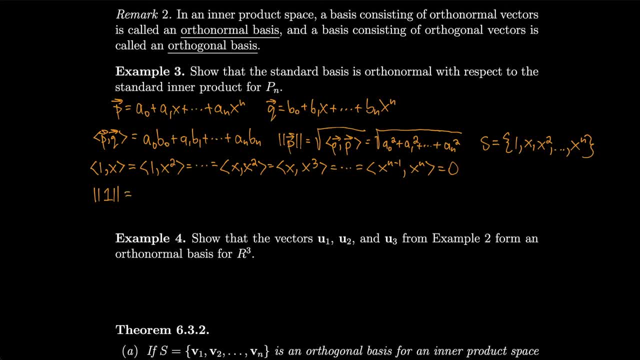 So that's going to be 1.. But if you take the coefficient on x and then you take the square root there- that's this one over here- Then again square root of 1 squared is 1.. So x has length 1 also. 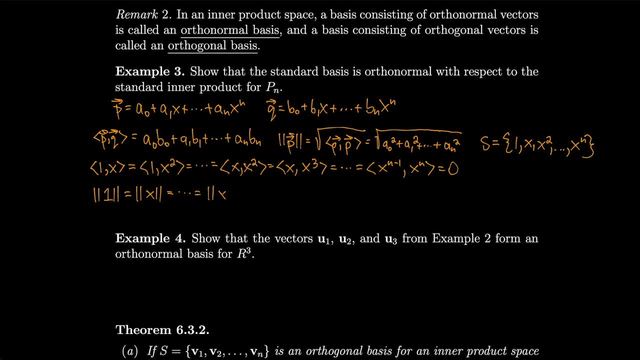 And similarly all the way through To x, and they all have length 1, because their coefficients are all 1.. They're all equal to the square root of 1 squared, So they all equal 1.. So these two facts imply that s is in fact orthonormal. 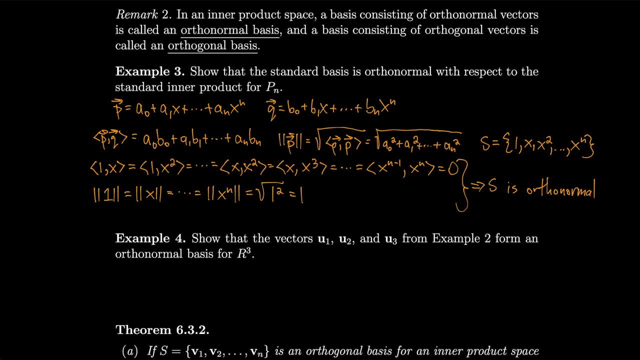 Because each vector is orthogonal to the others and they all have length 1.. Let's next show that the vectors u1, u2 and u3 from example 2 form an orthonormal basis For our three. So by example 2.. 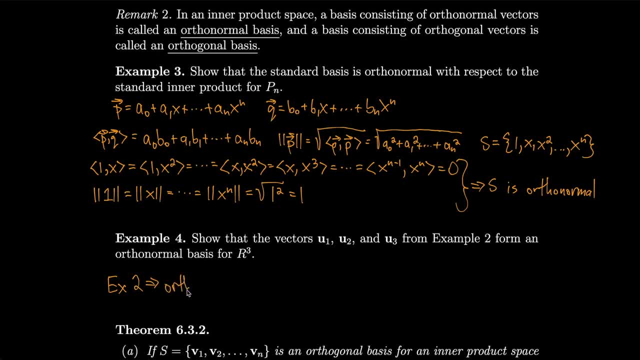 We saw that the set was orthonormal And that implies that the set is linearly independent. But we have a linearly independent set of vectors And there's three of them, So it has to be a basis Because, since the dimension of r3 is equal to 3.. 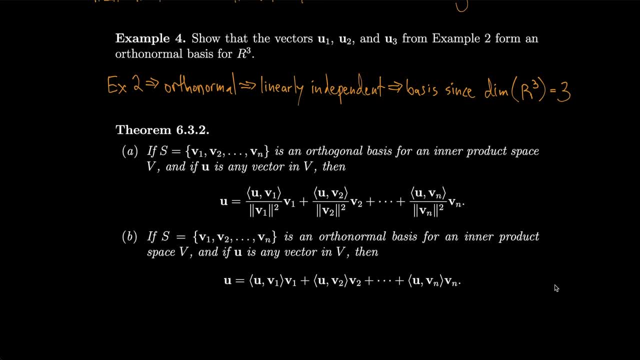 If s equals v1 through vn is an orthogonal basis for an inner product space v, And if u is any vector in v, Then u can be an orthonormal basis. So u can be written as the inner product of u with v1, u of v2, u through vn divided by. 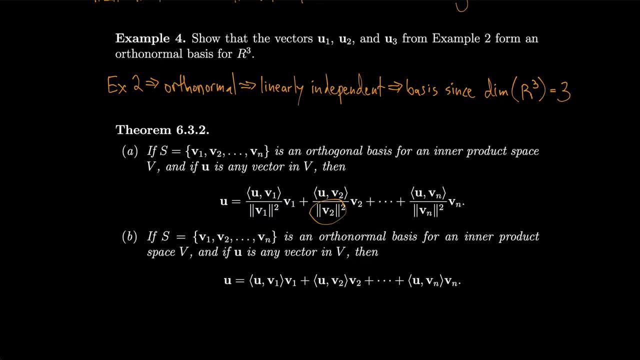 The length of v1 squared, length of v2 squared, length of vn squared, and so on, Multiplied by v1, v2 through vn. So you should notice, basically what we're doing is we're scaling these basis vectors In order to come up with a 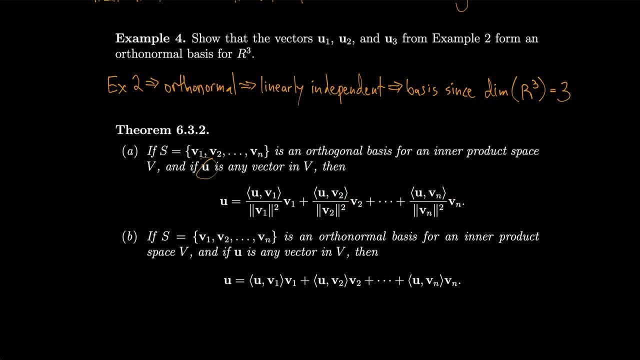 Particular vector u and v. If s equals v1 through vn is an orthonormal basis for inner product space v, And if u is any vector in v, Then u is equal to The inner product of u with v1 times v1, plus inner product of u with v2, and so on. 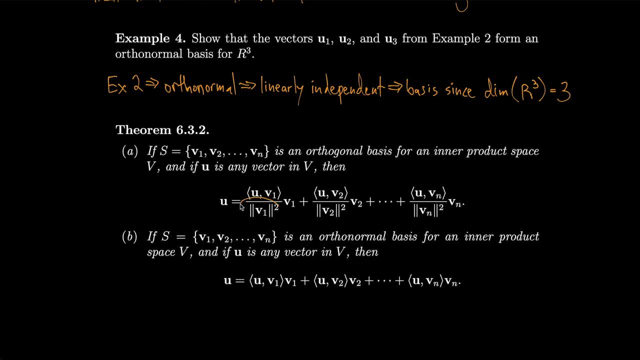 So if it's an orthogonal basis, notice we have to divide by lengths, Which should make sense. We have to normalize each of those vectors, v1 through vn, But if the basis is orthonormal, then we don't have to divide by anything. 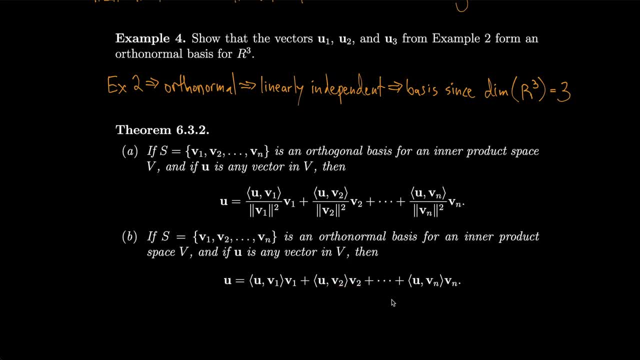 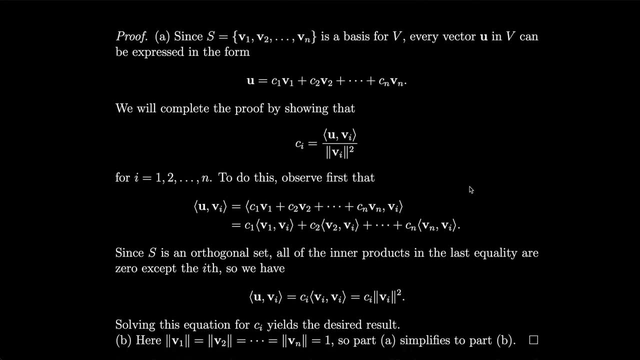 We just have to take a bunch of inner products. So let's prove this real quick. Since s equals v1 through vn, is a basis for v, Every vector u and v can be expressed in the form Where we have v1 through vn and some linear combinations. 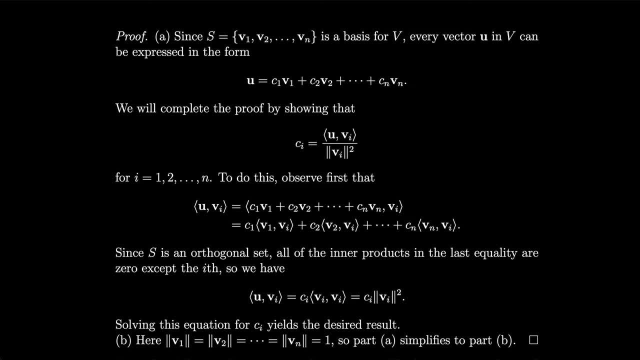 So a bunch of constants times. each of those Vectors will complete the proof by showing that the constants happen to be These inner products divided by these lengths. to do this, Let's observe first that the inner product can be rewritten as this dot product. 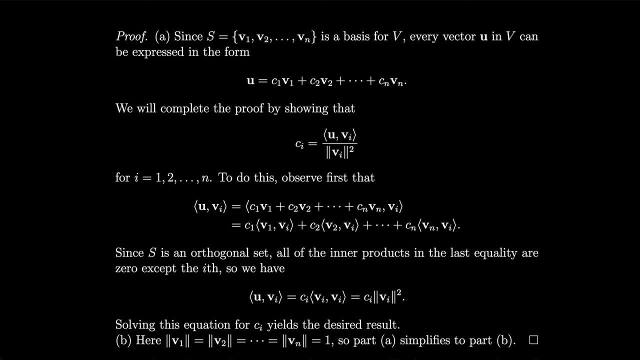 Taken as an inner product with v I, because that's what you is. you is just as linear combination. I just replaced it So we can use the properties of inner product to separate out all the constants And split up All of these into a bunch of separate inner products. 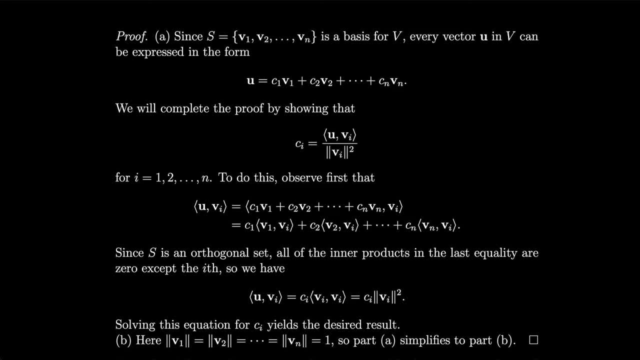 Since s is an orthogonal set, all of the inner products in the last equality are 0. Except for the i'th. So we have that the inner product with u of vi is equal to ci vi, vi, And that's the same thing as saying that this thing is the length squared. 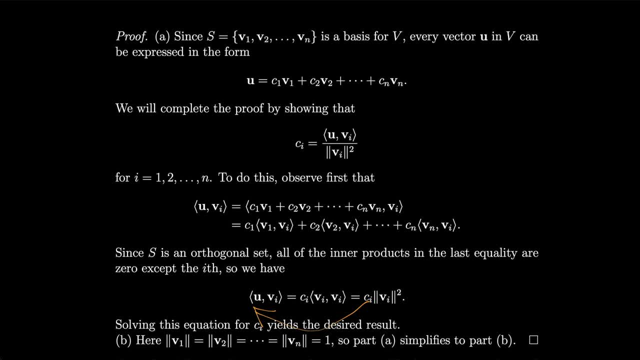 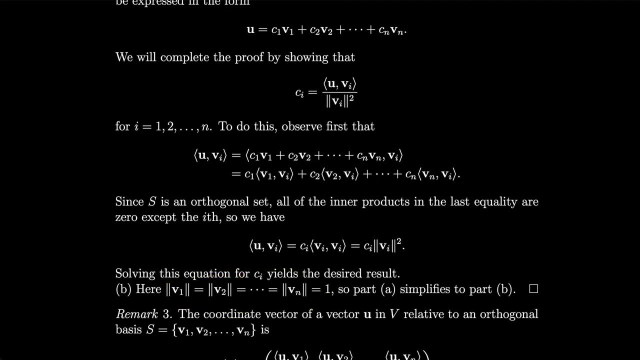 Then just Divide by vi squared and you get that ci is equal to this thing, Which is exactly what we wanted to prove. Let's do part b Here we have: each of the lengths is equal to 1.. So part a basically becomes part b. 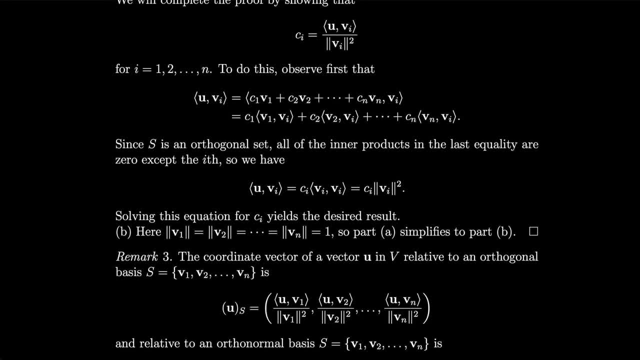 When you have an orthonormal set, we get part b for free, basically The coordinate vector of a, vector u and v relative to an orthogonal basis. s Is Just basically That Thing we just talked about And relative to an orthonormal basis. 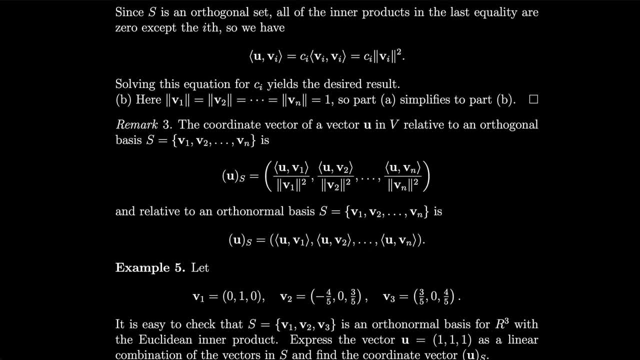 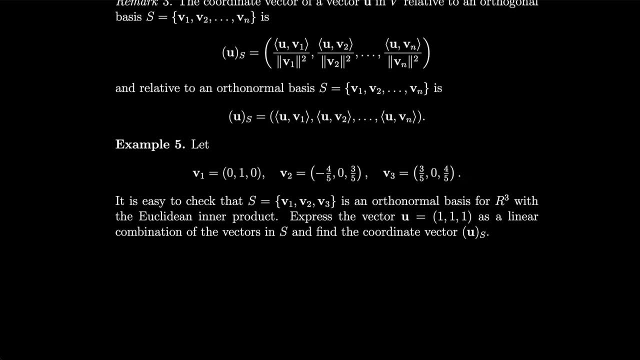 It's even simpler. How about we do an example? Let's let v1, v2 and v3 be the vectors given. It is easy to check that s equals v1, v2, v3 is an orthonormal basis for r3 with the Euclidean inner product. 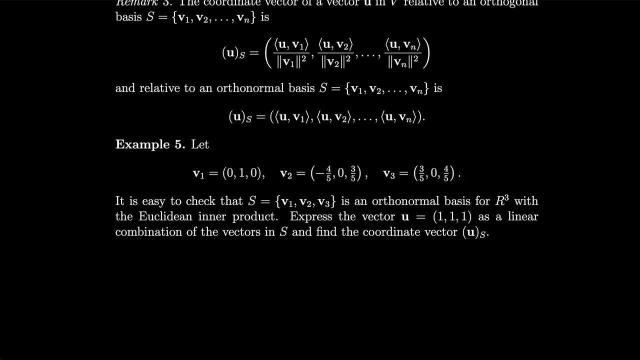 Express the vector u equals 1.. 1, 1, 1 as a linear combination of the vectors in s and find the coordinate vector u s. So let's get the inner product of u with v1, v2 and v3.. So the inner product of u with v1.. 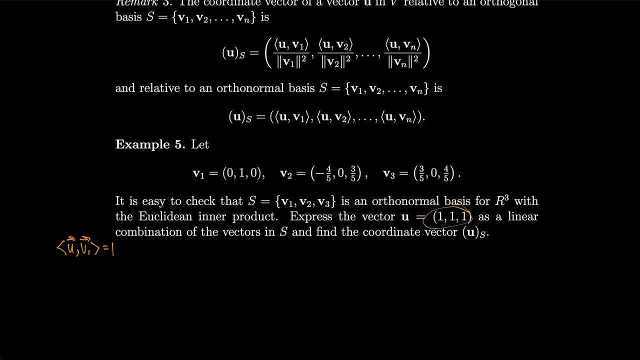 Well, that's just one right, because we have 1 1, 1 inner product. with v1, the zeros cancel most of the terms And we're Going to next do u with v2.. So with v2, we get negative 4 fifths times 1 plus 3 fifths times 1.. 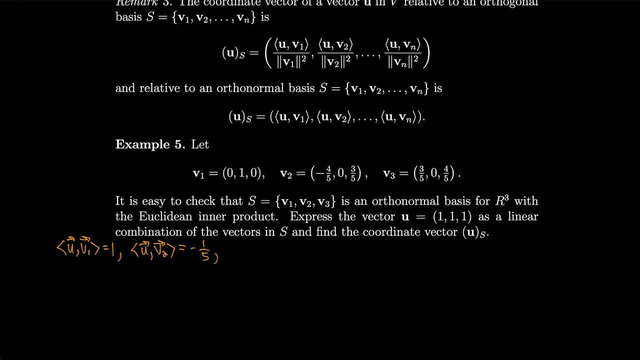 So we get negative 1 5th, All relative to the Euclidean inner product. And last but not least, Let's get u with v3.. So 3 fifths and 4 fifths gives us 7 fifths. Next let's use our formula to rewrite u. 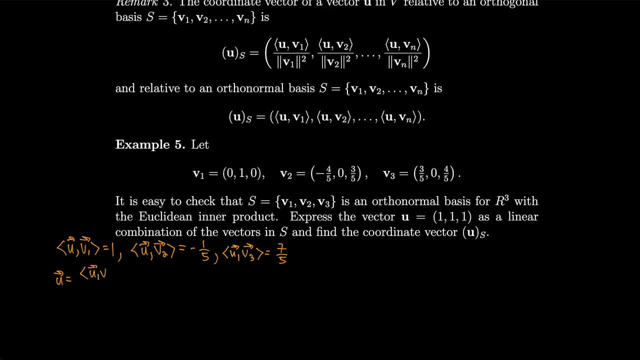 So we'll get that u is the inner product of u, with v1 divided by the length of v1 squared. That's supposed to be a comma and That'll multiply by v1 and then we'll add that to the inner product of u, with v2 divided by the length of v2 squared. 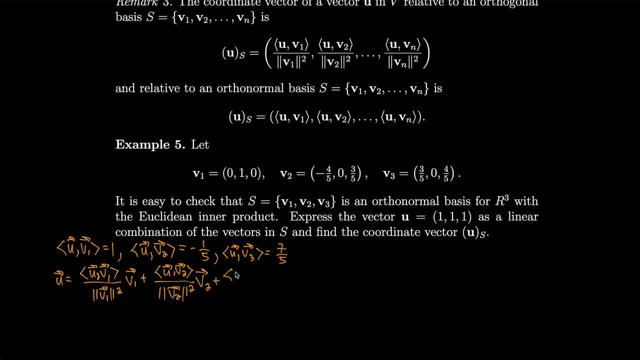 And multiply that by v2 and add that to the inner product of u with v3. Divide that by the length of v3 squared and multiply by v3. So that means that u is equal to just v1, because this inner product is 1 and the 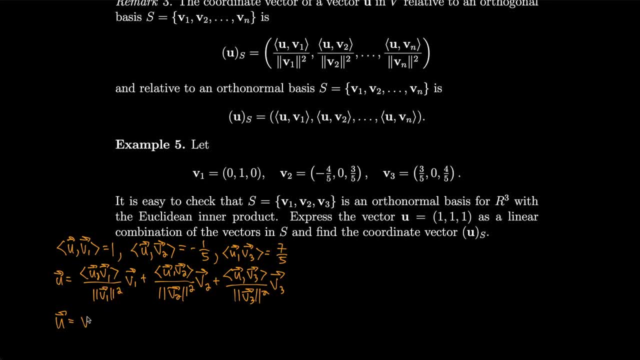 length of v1 is just 1.. So we just take 1 times v1.. This entire thing is 1, and then this is minus 1, 5th, and then dividing by the length of v2.. That's just 1.. 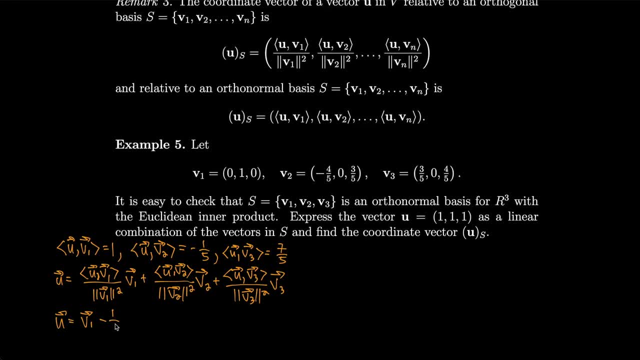 So we just get minus 1 5th. And then, lastly, we just get 7 5ths for v3, the coefficient Okay, so that's nice. That means that if I want to rewrite the vector 1, 1, 1,. 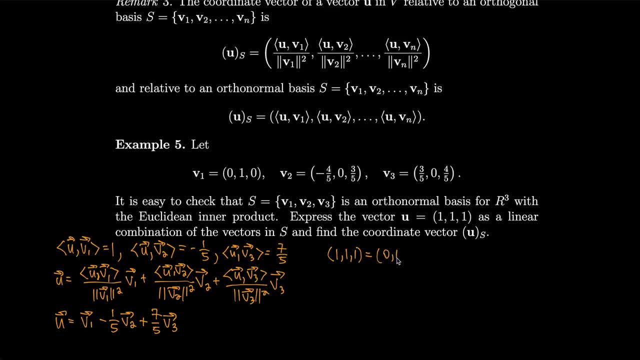 then that'll be v1, which is 0, 1, 0 minus 1 5th of v2, which is minus 4 5ths, 0 5ths, and add that to 7 5ths of v3,. 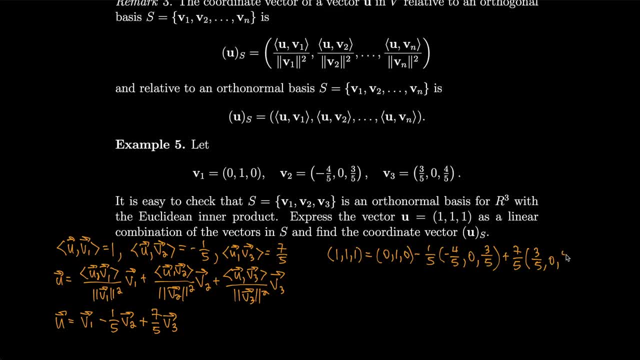 which is 3 5ths, 0, 4 5ths, as given in the problem, And we can. we can write the coordinate vector u s as the inner product of u with v1 in the first coordinate and inner product of u with v2. 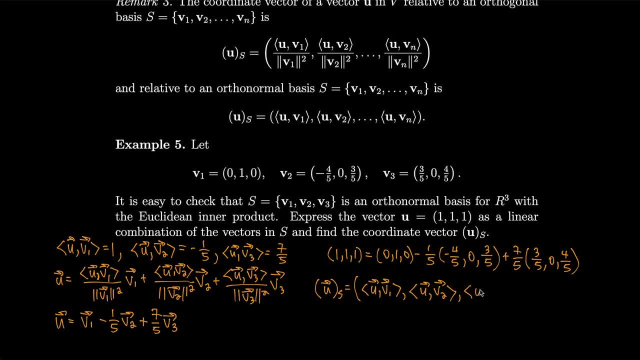 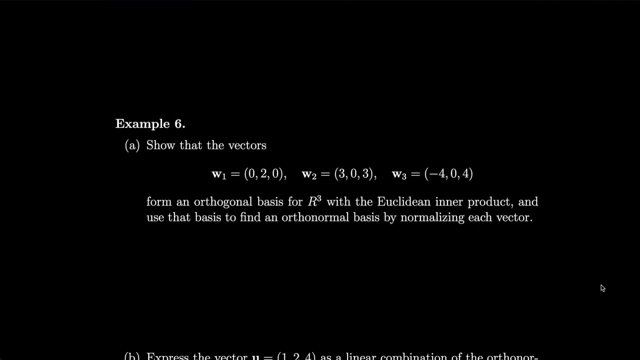 in the second coordinate and the inner product of u with v3 in the last coordinate. So that's just as we calculated: 1 minus 1, 5th, 7, 5ths. How about we do another example: Let's show that the vectors given form an orthogonal basis. 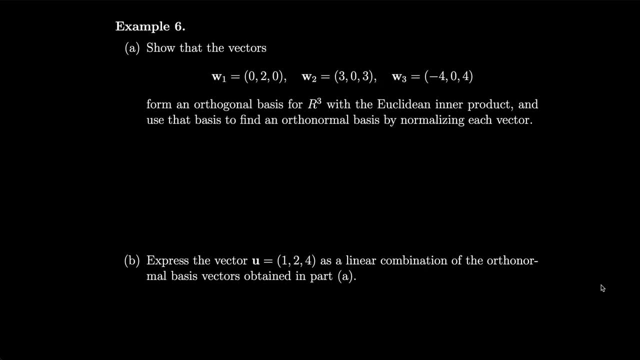 for our three with the Euclidean inner product And let's use that basis to find an orthonormal basis by normalizing each vector. So first let's get the inner products. We got w1 with w2.. Notice that'll be 0 because of these zeros and this 0.. 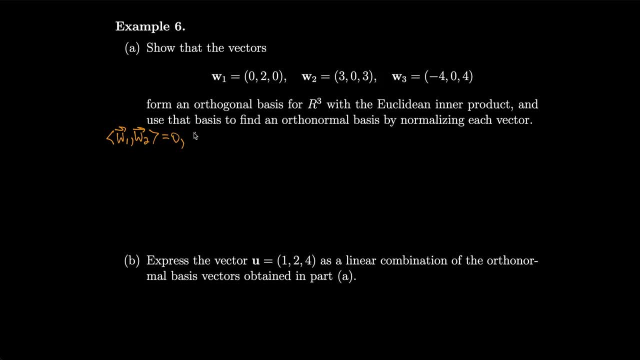 So that's 0.. Inner product of w1 with w3 is similarly 0. And inner product of w2 with w3 is also 0. Could have just written: them: all equal to each other equals 0. But in any case this implies: 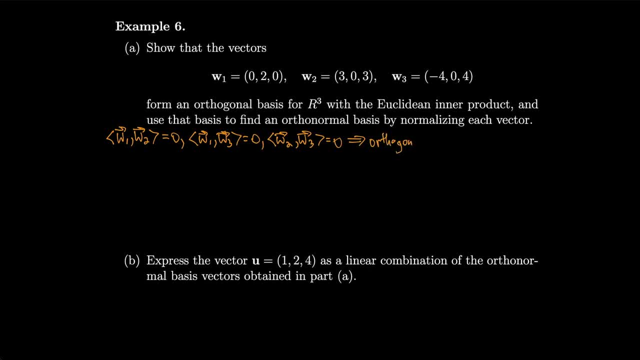 these vectors are orthogonal And that implies that the vectors are linearly independent, So they form a basis. So we just need an orthonormal basis. We have an orthogonal one right now. We can get an orthonormal one by dividing each vector by its length. 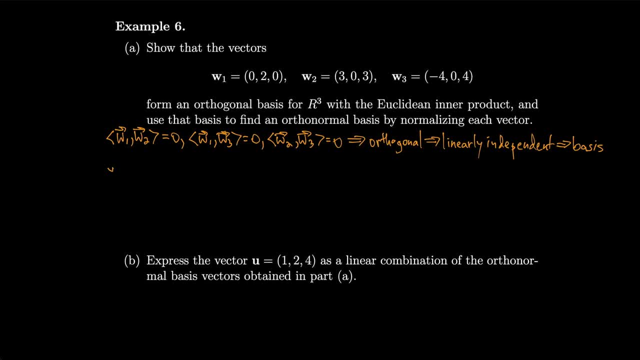 and normalize it. Normalizing them, making them all length 1.. So we can get our new vectors for our orthonormal basis, v1 equal to w1 divided by the length of w1. And that'll be 0, 2, 0 divided by the length of w1, which is 2.. 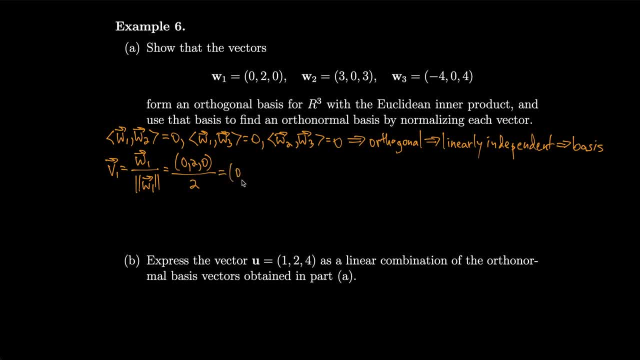 Just take the square root of 2 squared, So that's 0, 1, 0.. Let's get our next vector, v2.. Now by taking w2 and dividing that by its length, So that'll be 3, 0,. 3 divided by 3, rad 2,. 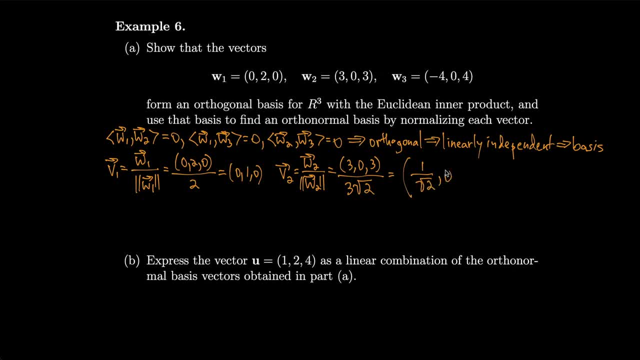 which is 1 over rad 2, 0,, 1 over rad 2.. Let's just get v3 now. So v3, is w3 divided by its length, So that's minus 4, 0, 4 divided by 4 rad 2.. 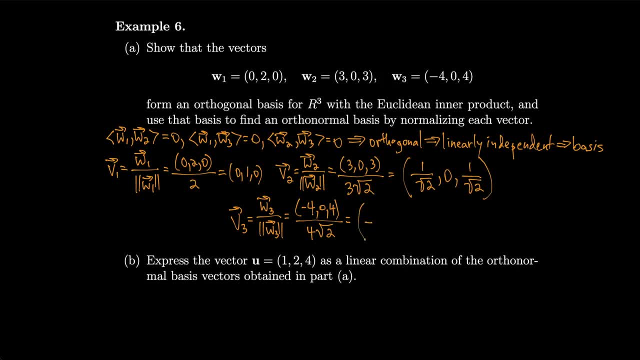 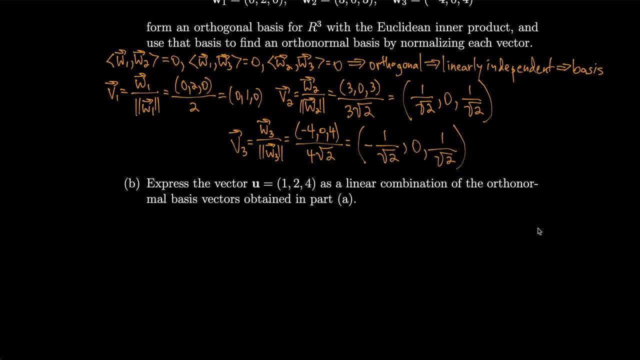 And that's equal to minus 1 over rad 2, 0, 1 over rad 2.. Next, how about we express the vector u equals 1 over rad 2.. to 4 as a linear combination of the orthonormal basis vectors. 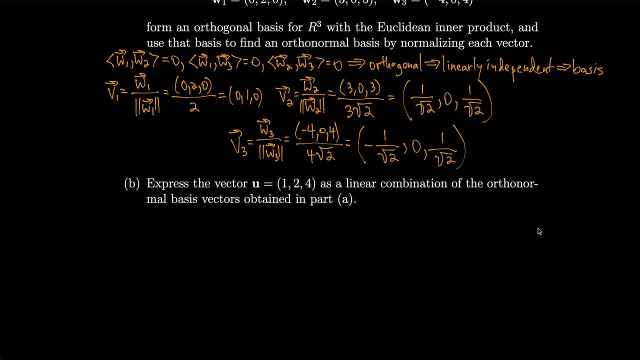 that we just got. So first we'll have to write u equal to each of those inner products scaling the basis vectors. So that's u with v1 times v1 plus u. inner product with v2, scaling v2, plus inner product of u with v3, scaling v3.. 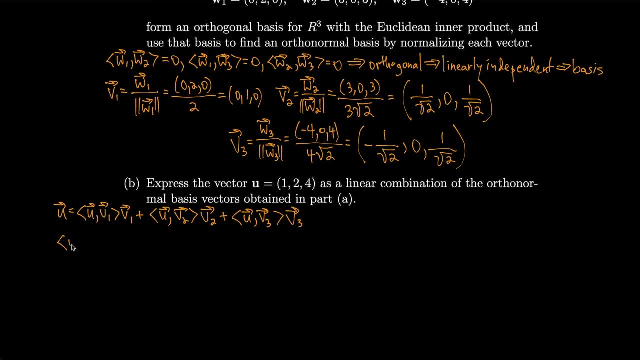 Okay, so let's calculate each of these inner products. So let's get: how about u with v1?? So that's equal to the inner product of 1, 2, 4 with 0, 1, 0. So that's just the dot product in this case. 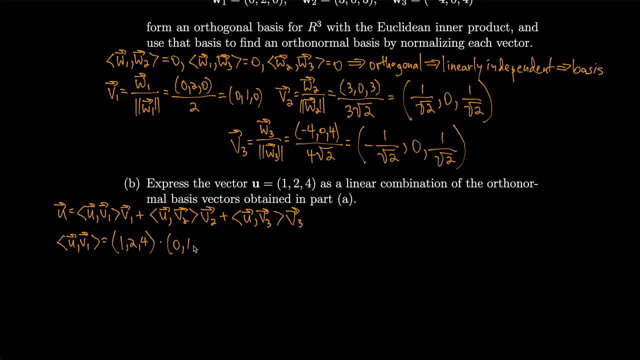 So 1,, 2, 4 dotted with 0, 1, 0.. So that's just the dot product in this case. So 1,, 2, 4 dotted with 0, 1, 0.. 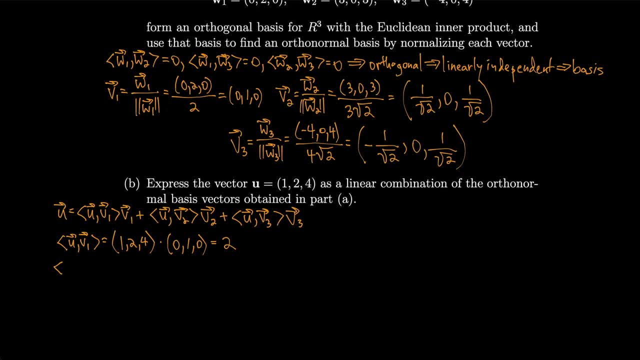 And that's just 2.. Let's get the other dot products. We need u with v2.. So we'll take 1, 2, 4 and dot that with 1 over rad 2, 0, 1 over rad 2.. 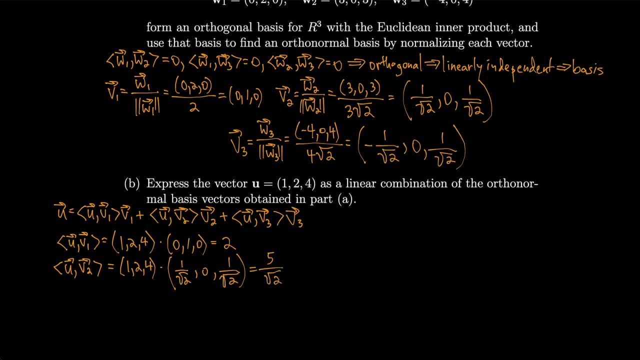 And we get 5 over rad 2.. Okay, one more. We'll get u with v3.. And that's just 1, 2, 4 dotted with minus 1 over rad 2, 0, 1 over rad 2.. 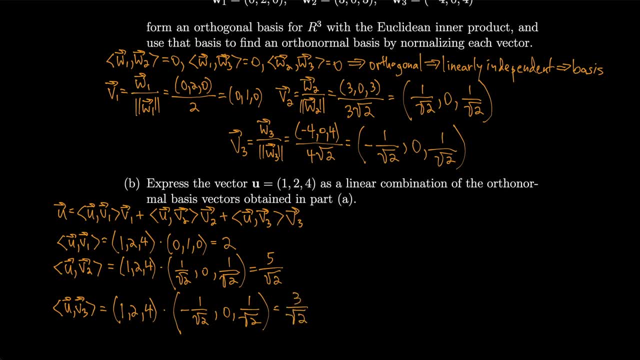 Which is 3 over rad 2.. So now we can take the vector 1,, 2,, 4. And we can rewrite it as 2 times v1, which is 0, 1, 0 plus 5 over rad, 2 times v2,. 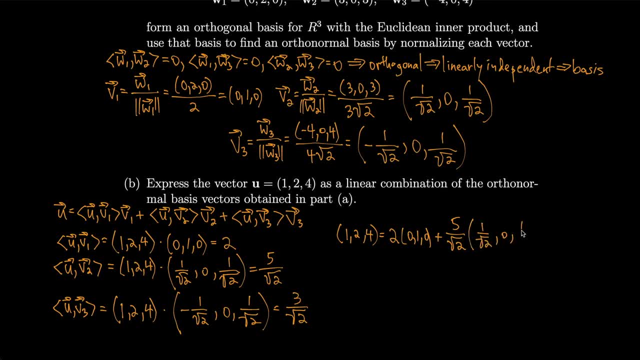 which was 1 over rad 2, 0, 1 over rad 2.. Plus 3 over rad, 2 times v1.. plus v3 minus 1 over rad2, 0, 1 over rad2.. Next up we have the projection theorem. 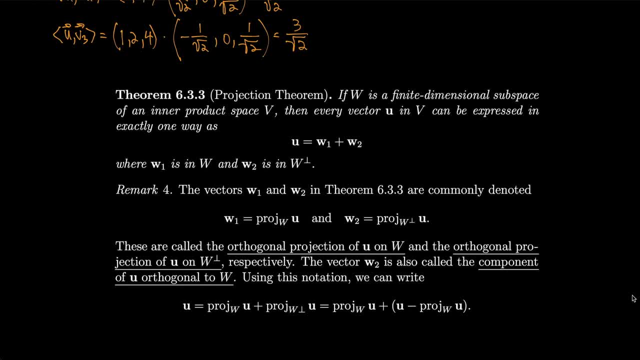 If w is a finite dimensional subspace of an inner product space, v, then every vector u and v can be expressed in exactly one way, as u equals w1 plus w2, where w1 is in w and w2 is in w perp. 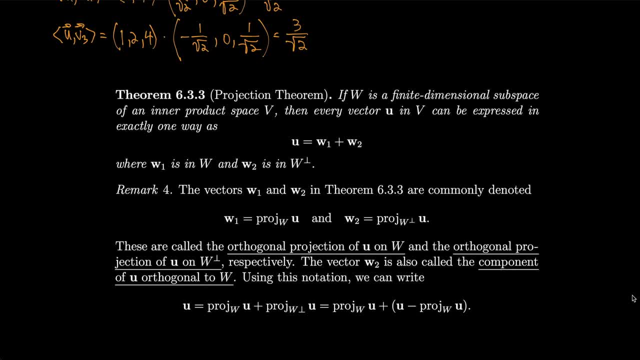 The vectors w1 and w2 in this theorem are commonly denoted as the projection of u on w and the projection of u on w perp. These are called the orthogonal projection of u on w orthogonal projection of u on w perp, respectively. 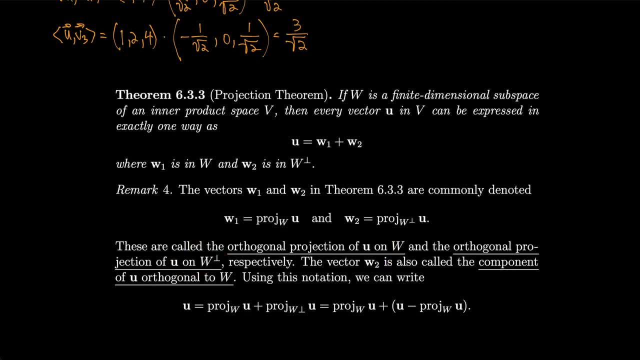 The vector w2 is also called the component of u orthogonal to w. Using this notation we can write u equal to w1 plus w2, but we'll just replace those with these guys And that's the same thing as writing. projection of u on w. 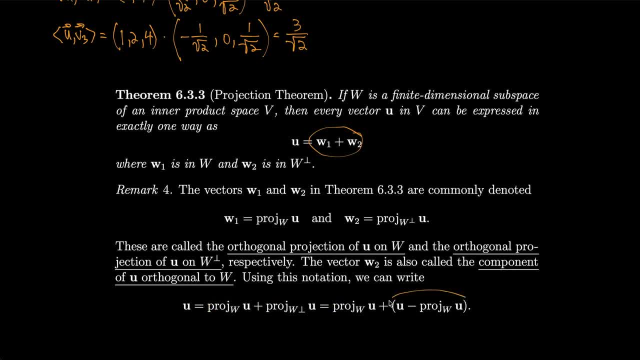 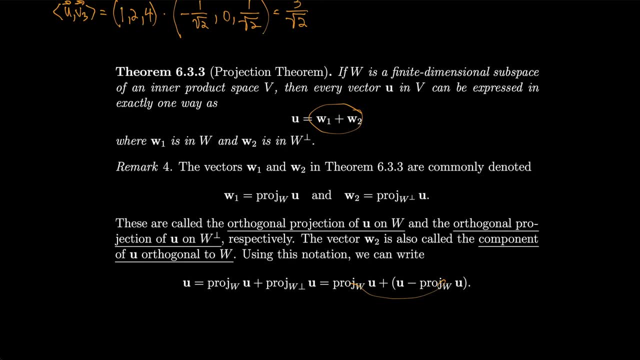 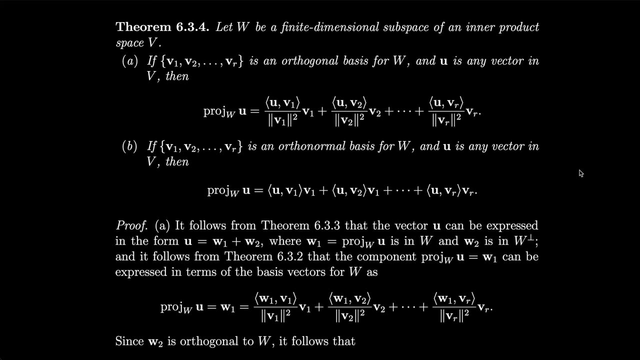 but replacing projection of u on w perp with u minus the projection of u on w. So you can see that these kind of cancel out. so it makes sense. Let w be a finite dimensional subspace of an inner product space, v. If v1 through vr is an orthogonal basis for w and u is any vector in v. 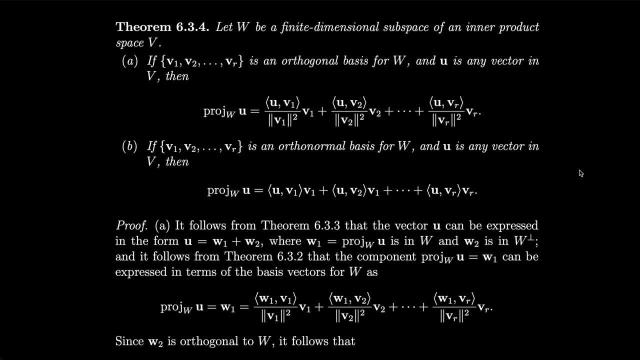 then the projection of u on w is equal to each of these inner products. Notice, this looks kind of familiar, right Divided by each of these lengths scaling each of the vectors, v1 through vr. If v1 through vr is an orthonormal basis for w, 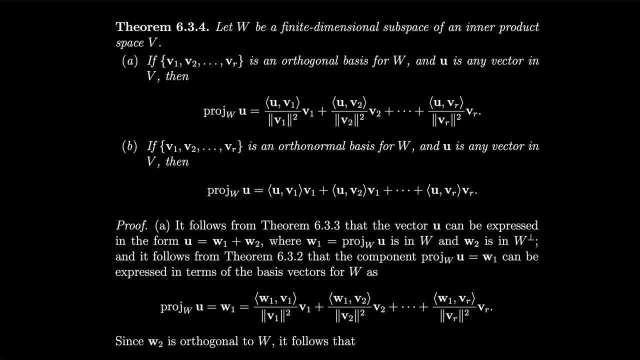 and u is any vector in v, then the projection of u on w simplifies, right. All of these are equal to 1, and they drop out. You just get the numerators times v1 through vr. Okay, let's prove this really quick. 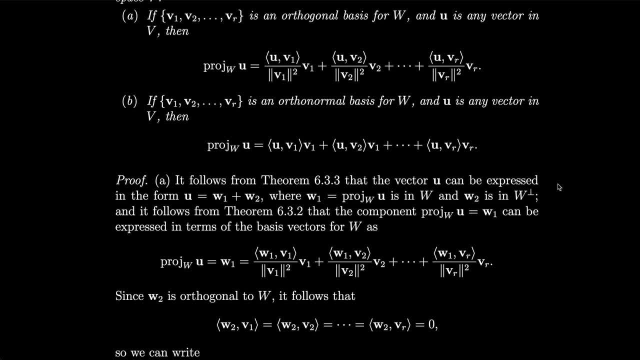 It follows from theorem 6.3.3 that the vector u can be expressed in the form: u equals w1 plus w2, where w1 is the projection of u on w and w2 is in w perp. It follows from theorem 6.3.2. 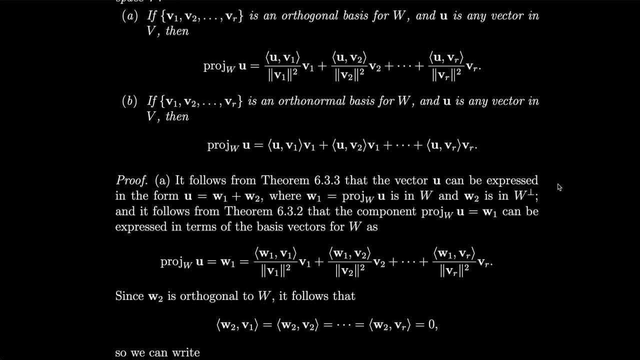 that the component projection of u on w equals w1 can be expressed in terms of the basis vectors. for w right, We can write it as w1, just because it's any vector we can rewrite in terms of the basis vectors. as long as we take all of these as the scalars. 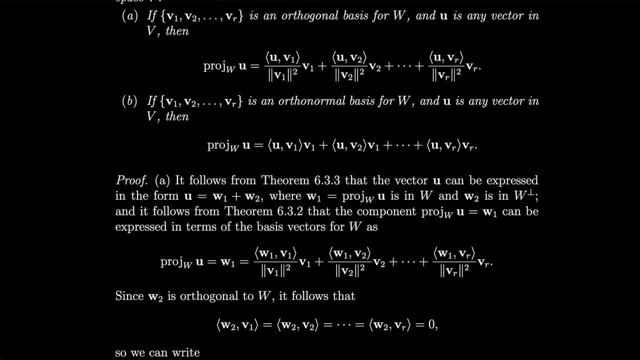 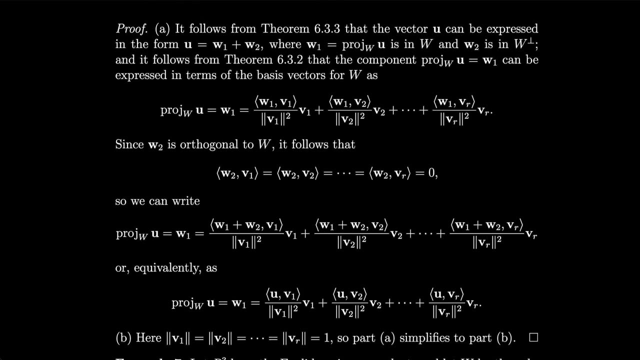 Since w2 is orthogonal to w, that means that if we take w2 and we look at the inner product with v1,, v2, et cetera, through vr, it must be 0. So therefore we can write that the projection of u on w 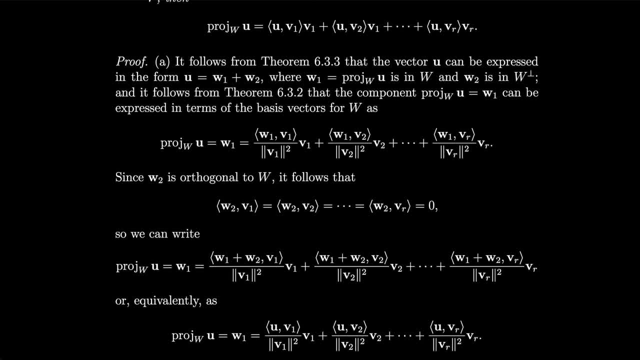 is equal to w1,. right This entire thing over here. But we can throw in all of these inner products in the numerator, because it's like adding 0 over and over, But that's the same thing as writing This thing right over here. 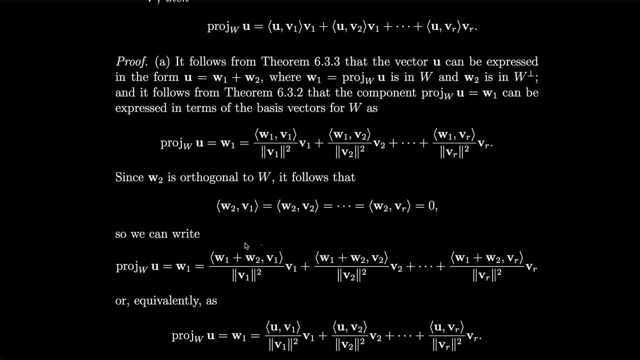 Basically, because of the orthogonality, we're able to throw in all of the w2 for free And when we add that to w1, we get u as we defined before. u is w1 plus w2.. Okay, perfect. 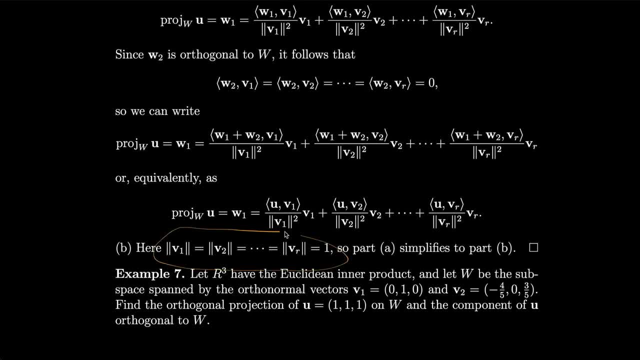 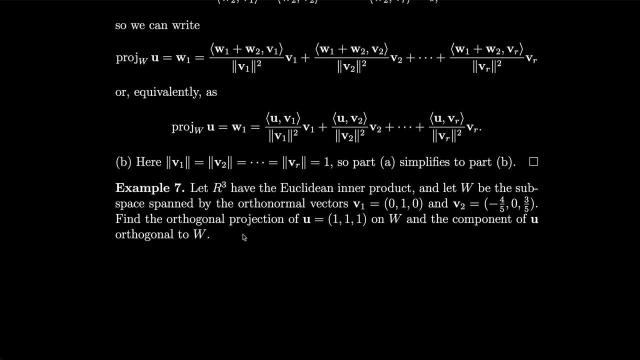 How about we let R3 have the Euclidean inner product and we'll let w be the subspace span by the orthonormal vectors v1, v2.. And let's find the orthogonal projection of u on w and the component of u orthogonal to w. 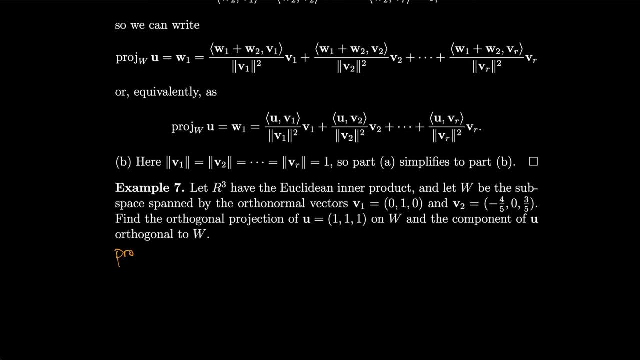 So first let's do the projection. So the projection of u on w will be equal to the inner product of u with v1 times v1, plus the inner product of u with v2 times v2.. So that's 1 for the inner product with u and v1. 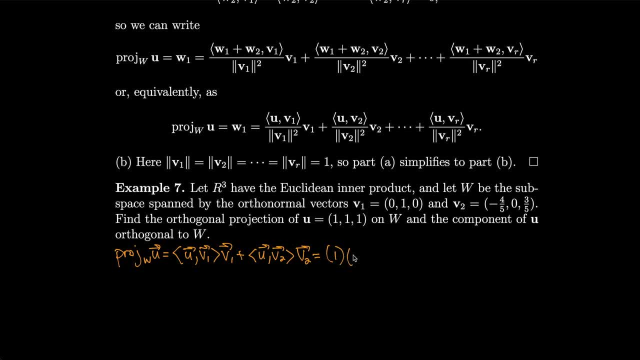 because it's just the dot product, Euclidean inner product, And we'll multiply that by v1, which is 0, 1, 0. And add that to the inner product of u with v2.. So that's minus 1.. 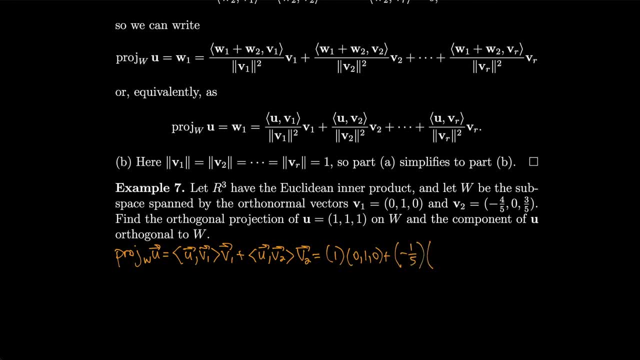 5th times. v2 is minus 4 5ths, 0, 3 5ths And we get 4: 20 5ths, 1 minus 3- 20 5ths. OK, let's get the component of u orthogonal to w. 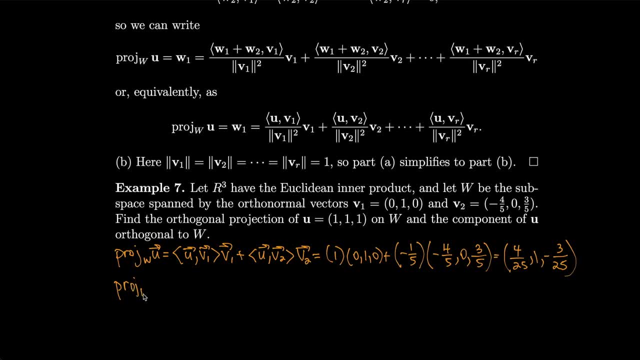 So that's the projection of u on w perp. don't like that perp? there we go. so that's going to be equal to u minus the projection of u 1 w. so that's 1: 1, 1 minus 4 over 25, 1 minus 3 over 25, and simplifying, we get 21 over 25, 0, 28 over 25. 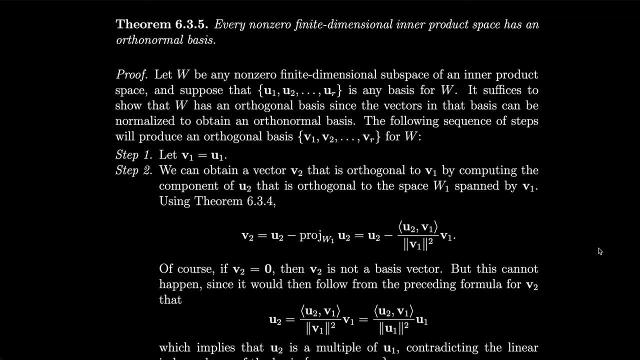 every non-zero finite dimensional inner product space has an orthonormal basis. let's see if we could prove this. let w be any non-zero finite dimensional subspace of an inner product space and suppose that u 1 through u r is any basis for w, it suffices. 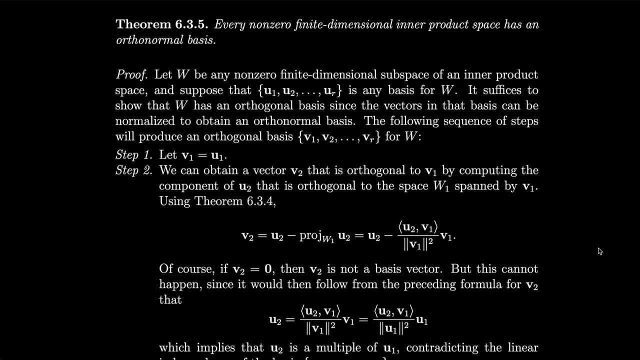 to show that w has an orthogonal basis, since the vectors in that basis can then be normalized to obtain an orthonormal basis. so all we gotta do is find an orthogonal one. the following sequence of steps will produce an orthogonal basis for w. so this proof is actually kind of. 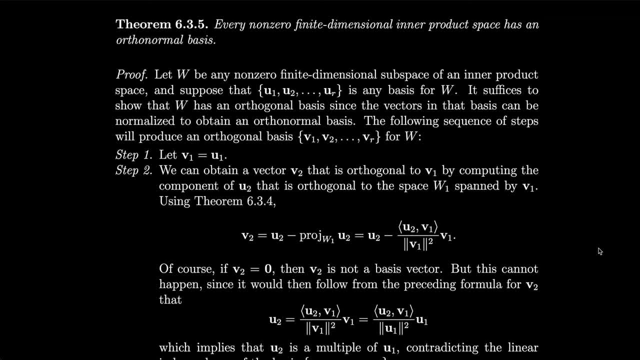 important because these steps are exactly what we'll use to find orthogonal basis and then we'll normalize them to get orthonormal ones. step one: let our first vector in our new basis, v1, be equal to our first old vector, u1, from the old basis. step two: let's obtain a new vector. 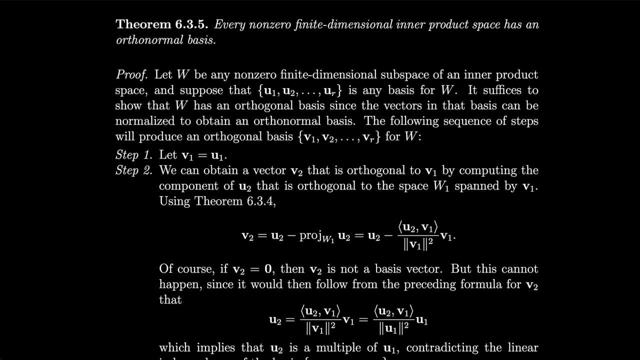 v2 that is orthogonal to v1, by computing the component of u2 that is orthogonal to the space w1 spanned by v1. so, using theorem 6.3.4, v2 is u2 minus the projection of u2 and w1 to the space w1. 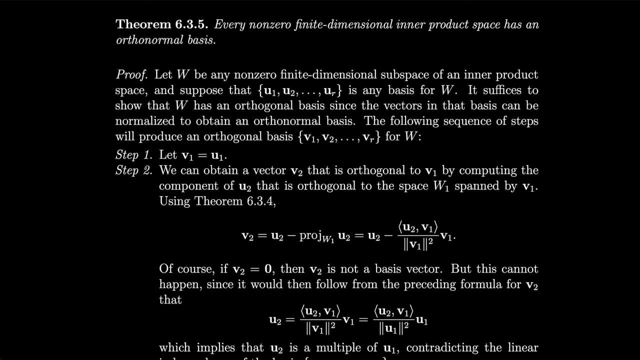 spanned by v1. so using theorem 6.3.4, v2 is u2 minus the projection of u2 and w1. so using theorem 6.3.4 w1, so u2 is v2 is u2 minus the inner product of u2. v1 divided by length of v1, squared times v1. 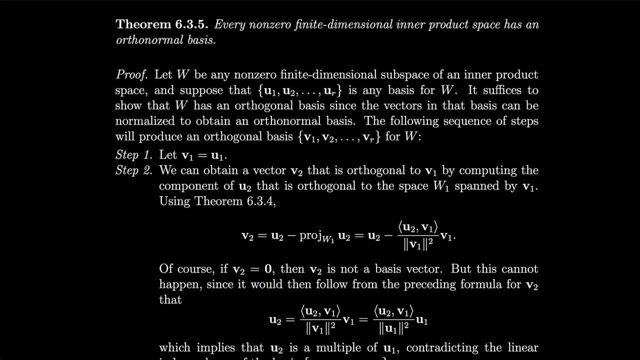 if v2 is 0, then v2 is not a basis vector. but this can't happen, since it would then follow from the preceding formula for v2 that u2 would equal this entire thing. right, but then that would be equal to the entire thing times u1 divided by length of u1 squared. 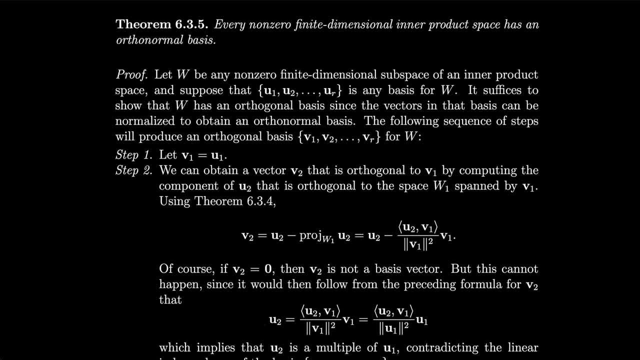 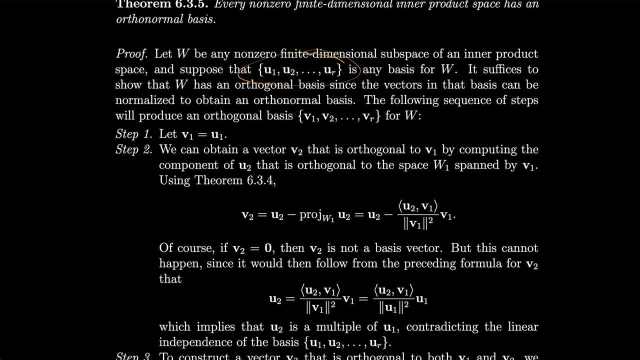 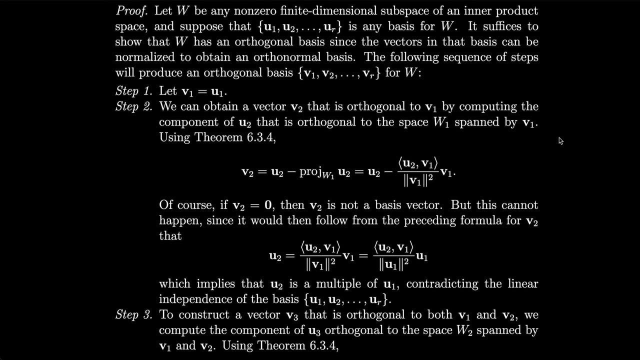 but then u2 would have to be a multiple of u1, but they can't be because all of the u's are linearly independent- one of the nice things about starting out with a basis to begin with. next step, we want to get a vector v3 that is orthogonal to both v1 and v2. so what we do is we compute the component of v. 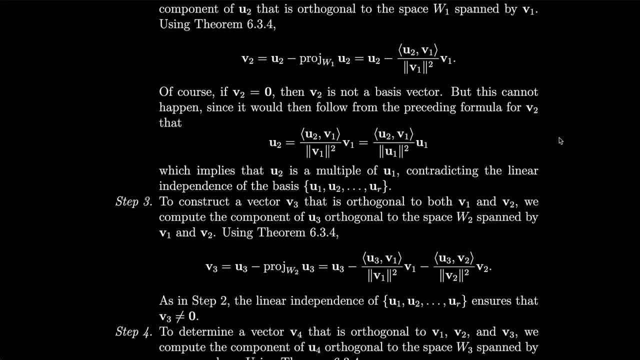 orthogonal to the space w2 spanned by v1 and v2. so that means that that v3 would be the u3 minus the projection of u3 on w2. so that means that we would have to take u3 minus the inner product of u3, with v1 divided by v1 squared times v1 minus inner product of u3, with 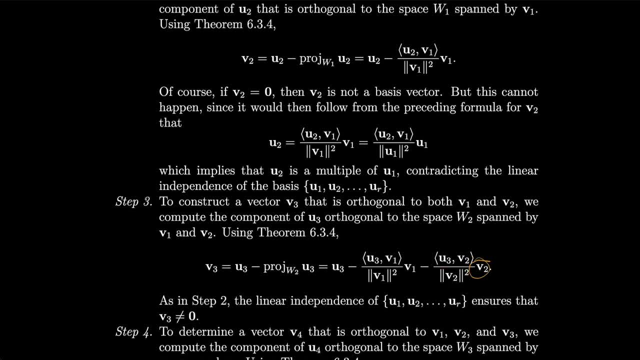 v2 divided by v2, squared v2. so each time that you want to get another vector, you're doing another step. you have to subtract more and more other vectors. you have to do more and more inner products, because you have to make sure that it's orthogonal to every other vector in the set, so as 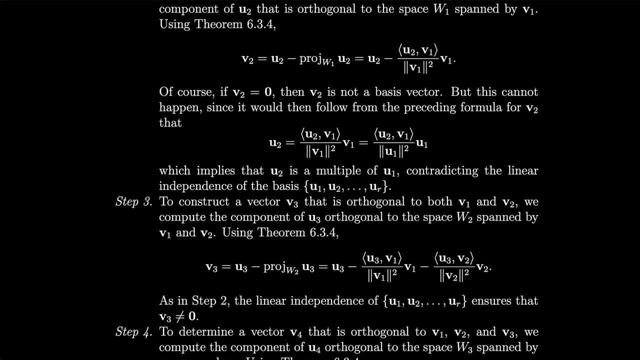 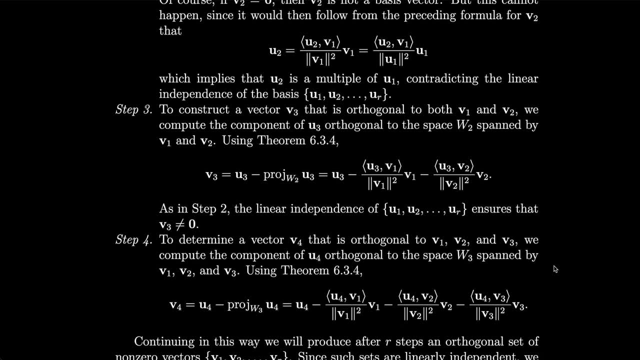 in step two: linear independence of the original basis vectors: ensure that v3 will not be equal to zero. to determine a vector v4: again, keep in mind that v3 will not be equal to 0.. to determine a vector v4: again, keep in mind that v3 will not be equal to 0.. to determine a vector v4: again, keep in. 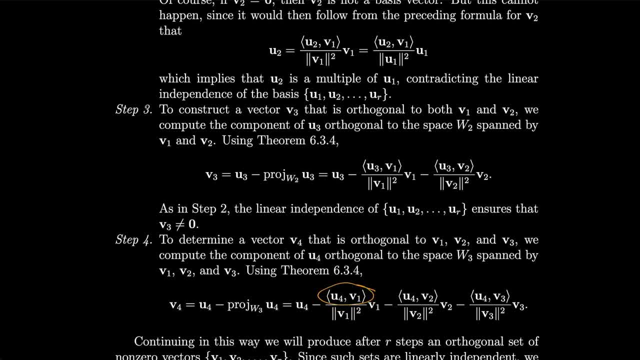 keep in mind that v3 will not be equal to 0.. to determine a vector: v4- again, keep going. this time you'll have to do u4 with v1, u4, v2, u4, v3, so you'll have to subtract off three of these guys. 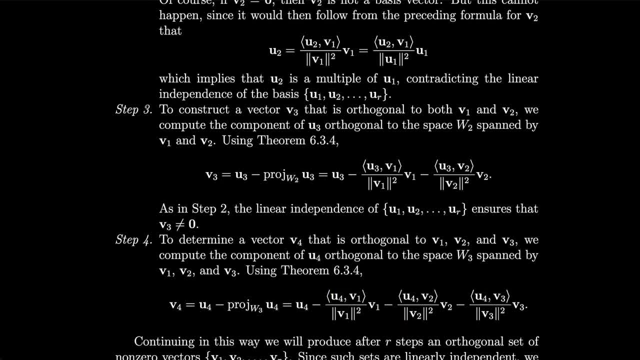 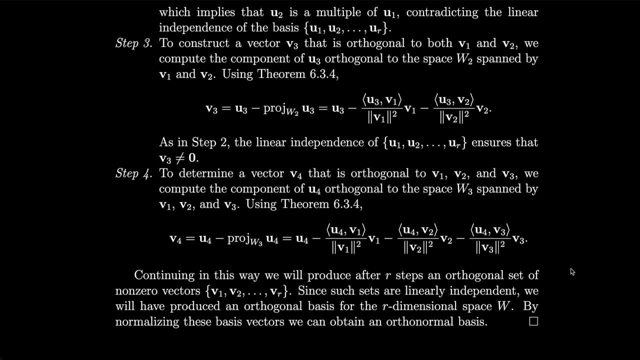 for v1, v2 and v3 to make sure that it's orthogonal to all of them. continuing this way, we will produce, after our steps, an orthogonal set of non-zero vectors, v1 through vr. since such sets are linearly independent. we will have produced an orthogonal basis for the r-dimensional space w, and then we 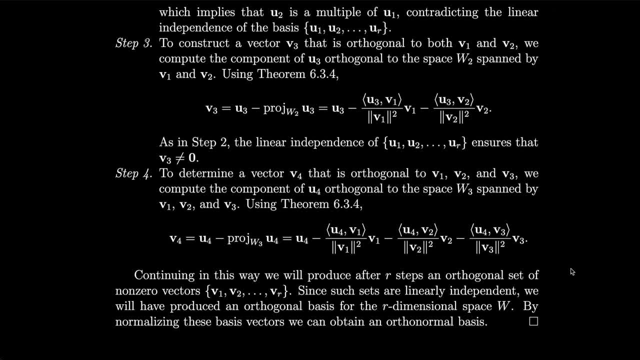 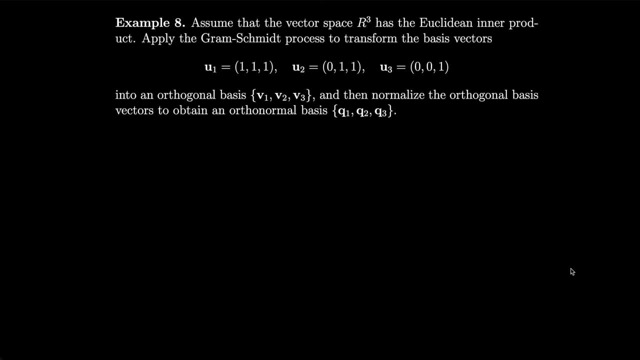 will produce an orthogonal basis for the r-dimensional space w, and then we can look, normalize them to obtain an orthonormal basis. just divide by the lengths. okay, let's do an example. how about we assume that the vector space r3 has the euclidean inner product? 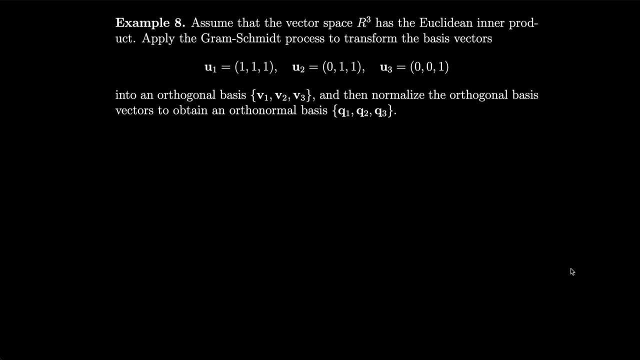 let's apply the gram schmidt process- that's the way that we proved the previous theorem- to transform the basis vectors u1, u2 and u3 into an orthogonal basis- v1, v2, v3- and then normalize the orthogonal basis vectors to obtain an orthonormal basis q1, q2, q3. 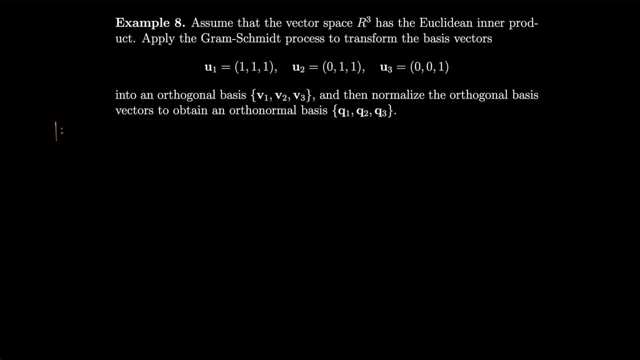 so let's do step one. let's first write v1, our new basis vector, equal to u1, so that'll just be one one one step two. now let's write v2, equal to u2, minus the projection of u2 on w1, so that'll be u2. 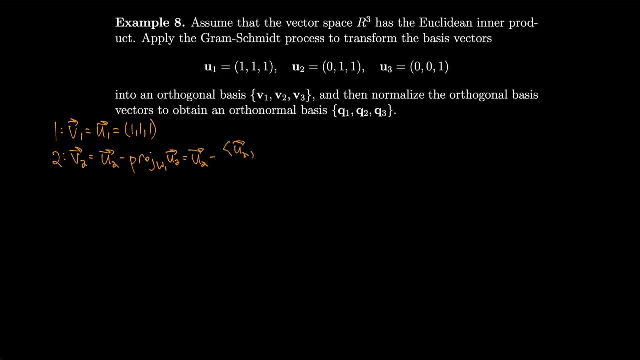 minus the inner product of u2, with v1 divided by the length of v1, squared times v1. so that's zero one one minus two thirds, one one, one right, because the uh inner product we get and that'll give us minus two thirds, one third, one third for v2. so we have two vectors down. 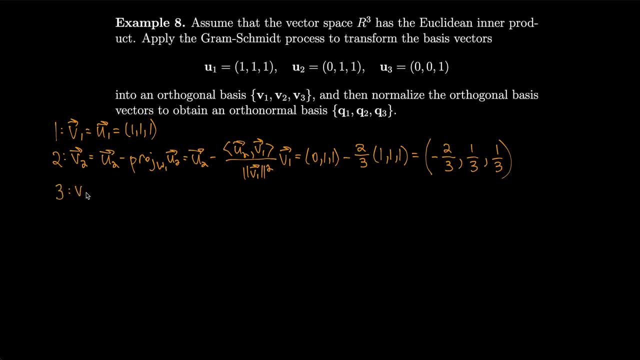 we just need one more. so step three: we have v3 equal to u3, minus the projection of u3 on w2, so that's u3 minus inner product of u3 with v1 divided by length of v1, squared times v1. but we also have to subtract off the inner product of u3 with v2. 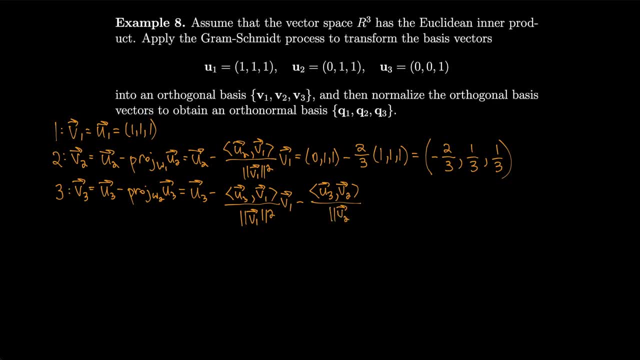 divided by the length of v2, squared times v2. okay, so that'll be equal to zero. zero one minus one third. one one. one minus one third. divided by two thirds times minus two thirds, one third, one third- and simplifying, we get zero minus a half half. 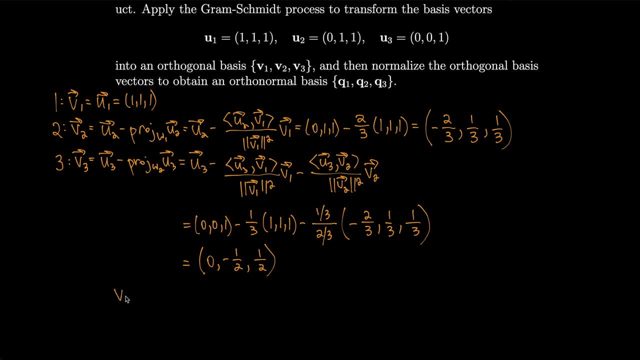 okay, great. so now we have an orthogonal basis where our vector v1 is equal to one one one, our vector v2 is equal to minus two thirds- one third, one third- and our vector v3 is equal to zero minus a half half. just to check now, we can get the length of v1 equal to square root of three, the length of v2. 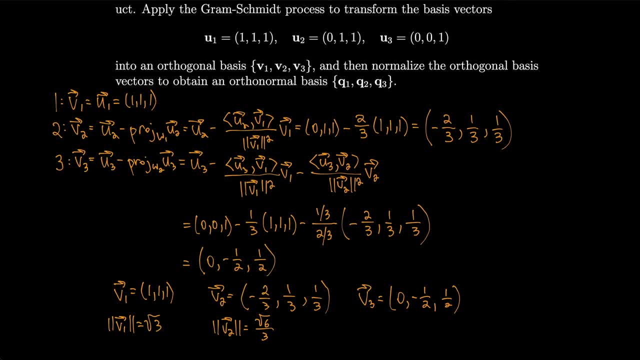 equal to square root of six over three and the length of v3 equal to one over rad two. so these vectors are not normal, they're not already normalized, they don't have length one. so in order to find the orthonormal basis, we're going to have to normalize. okay, so we'll write q1. 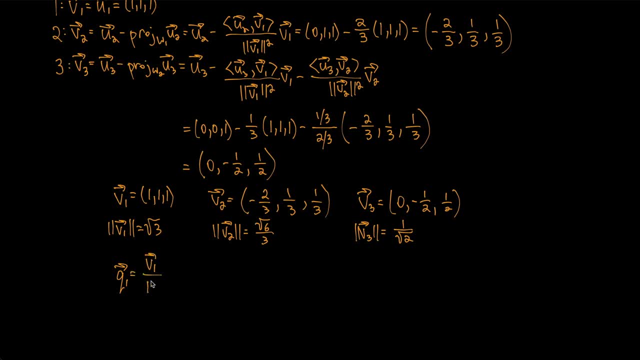 equal to v1 divided by its length. that'll be our first orthonormal basis vector. so that's one divided by rad three, one divided by rad three, one divided by rad three, all right q2 time. so that'll be v2 divided by its length. 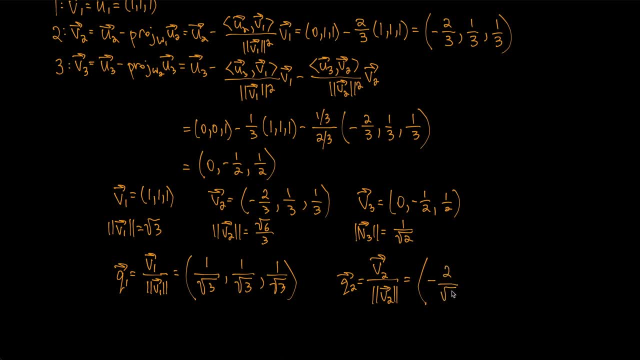 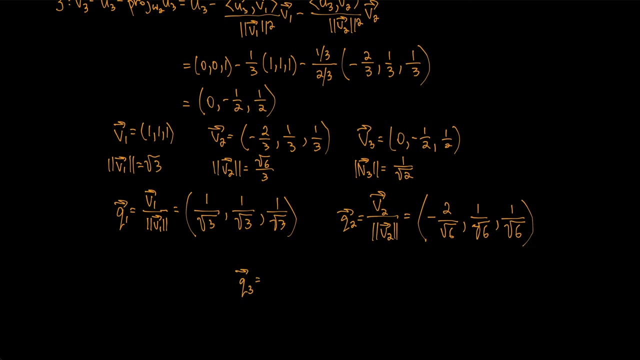 so that's minus two over radical six, one over rad six and one over rad six. lastly, how about we get q3? so that's v3 divided by the length of v3, and that's zero minus one over rad two, one over rad two, and that's our ethanol basis. 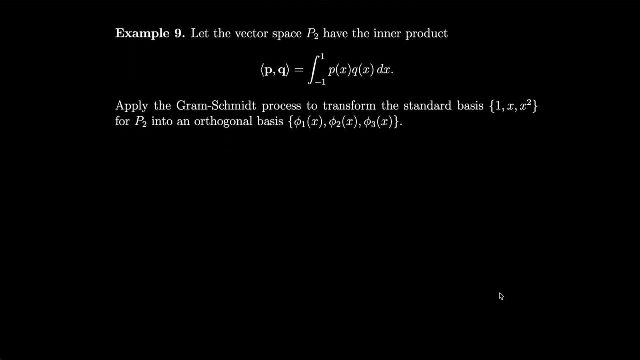 so we can calculate this by taking the two sides of the equation and we'll be left with p1 plus v2 plus v2 squared in the product, and that's the constant integral from one to one. okay, for our next example, how about we let the vector space p2 have the inner product over here, given by the integral? 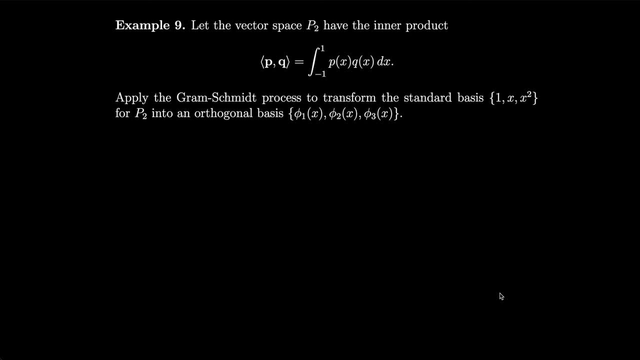 for minus one to one of the product. and let's apply the gram-schmidt process to transform the standard basis, one x, x squared on p2, into an orthogonal basis: v1, v2, v3, u1 equal to 1, u2 equal to x and u3 equal to x squared for our original basis. 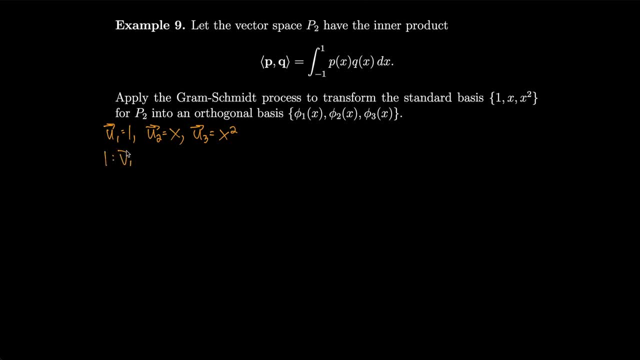 Let's apply step 1, and we'll set v1 equal to u1, and that's just the vector 1, the polynomial 1.. Okay, next let's get v2.. So what we'll do is we'll have to take the inner product of u2 with v1,. 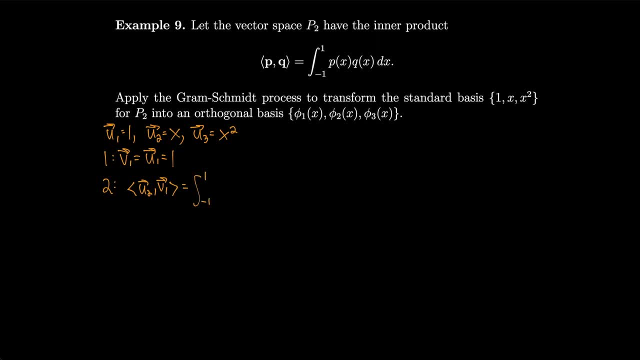 and that should be equal to the integral, from minus 1 to 1, of 1 times x, dx. And notice that's odd inside over a symmetric interval, so it's just 0.. Or you can do the antiderivative x squared over 2, plug in 1, subtract off. 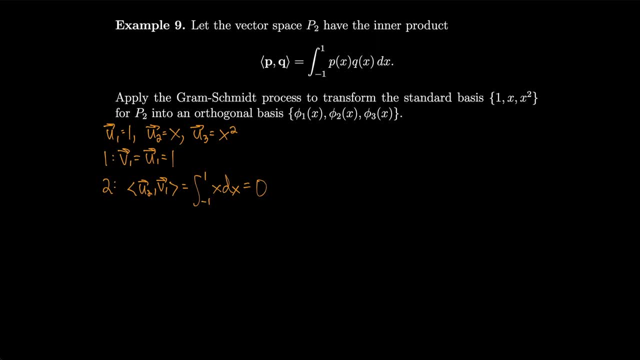 what you get. plug in minus 1, you'll get 0.. In any case, we have that v2 is equal to u2, minus the inner product of u2, with v1, divided by length of v1, squared times v1, and that's u2, so it's just x. 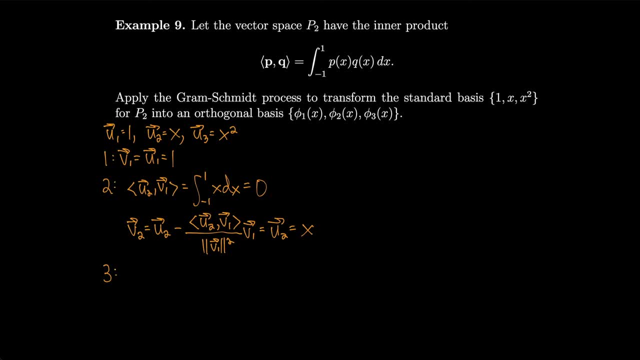 Cool, let's do 3.. For 3, we get, or let's just do u3, inner product with v1.. So that's the integral, from minus 1 to 1, of 1 times x squared dx. So that's x cubed over 3, evaluated from minus 1 to 1, when we do the antiderivative. 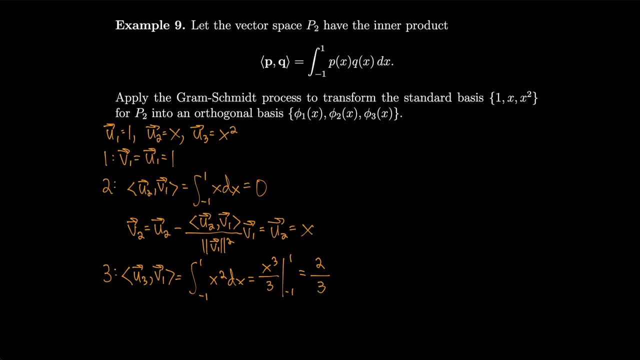 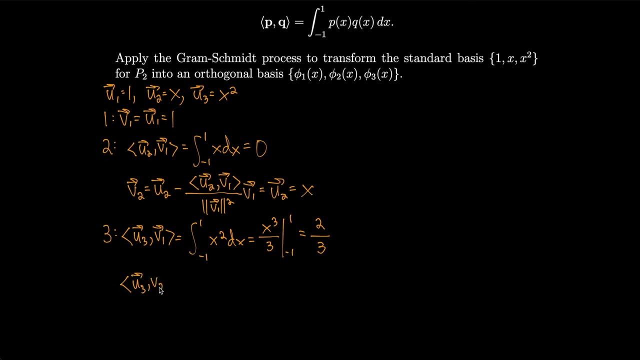 And plugging in 1 and minus 1 and subtracting, we get 2 thirds. Let's next get the inner product of u3 with v2.. So that's the integral from minus 1 to 1 of x cubed dx. 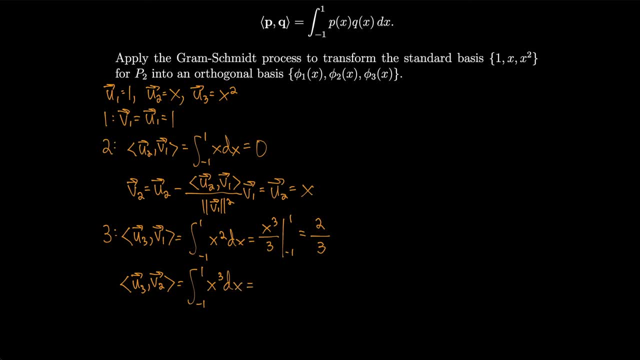 because it's x times x squared. So again, odd function, symmetric interval. or, if you want, I'll just write out the antiderivative x to the 4th over 4, from minus 1 to 1.. In any case, 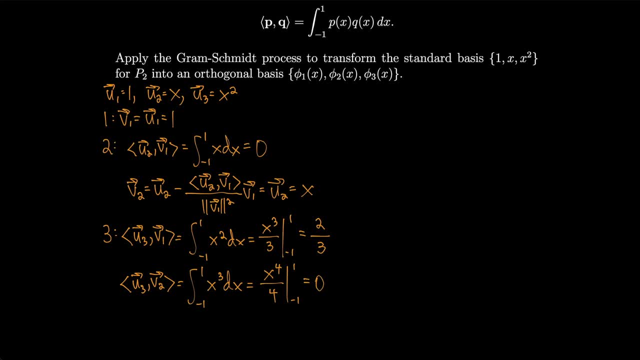 you should get zero Next up. let's get the length, So the length of v1 squared, that's the inner product of v1 with v1, which is the integral from minus 1 to 1 of 1 dx. Okay, so you could just do b minus a or take the antiderivative of 1,. 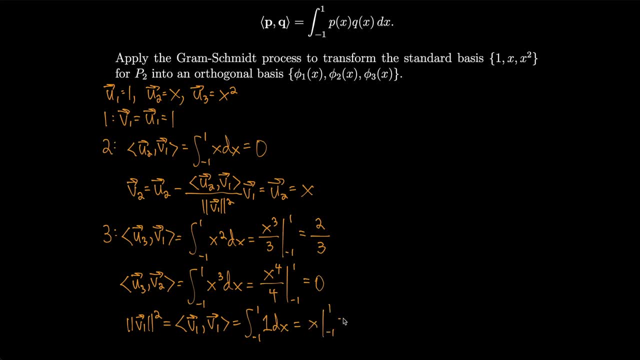 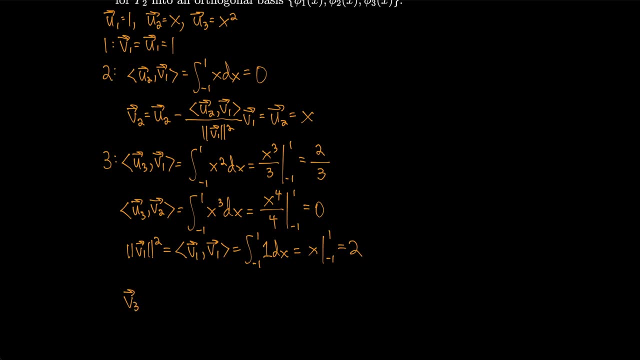 you get x from minus 1 to 1, in any case it's 2.. So now we can write: v3 equal to u3 minus the inner product of u3 and v1 divided by the length of v1 squared times v1 minus inner product of u3 with v2. 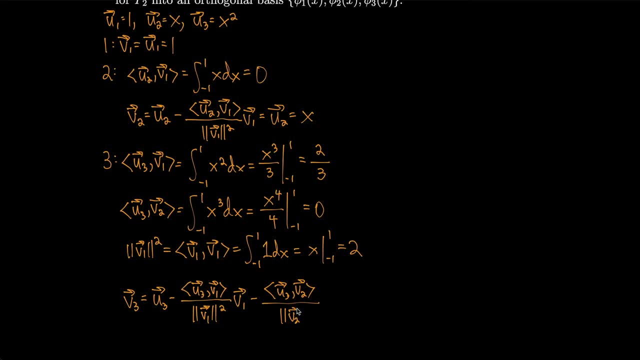 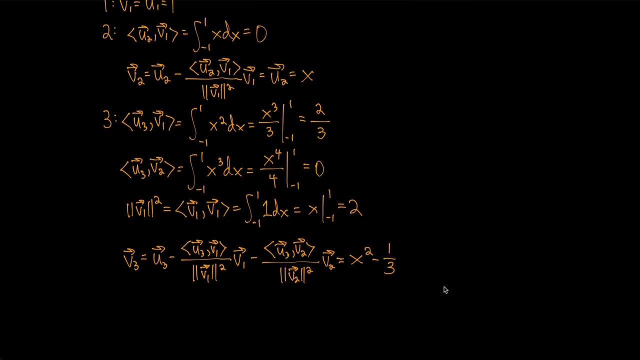 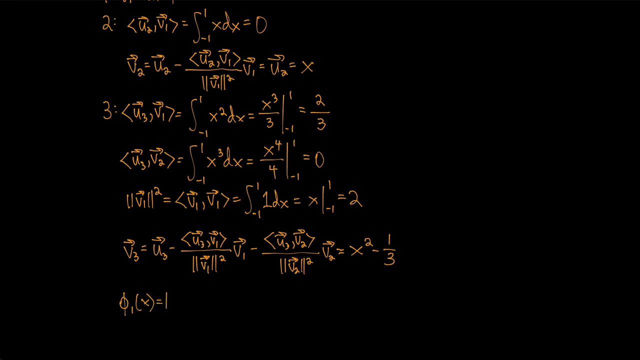 divided by the length of v2, squared times v2,, and you get x squared minus 1 third. just by plugging in everything, That would be 1.. Okay, so that means that v1 of x is just 1, as it was before. 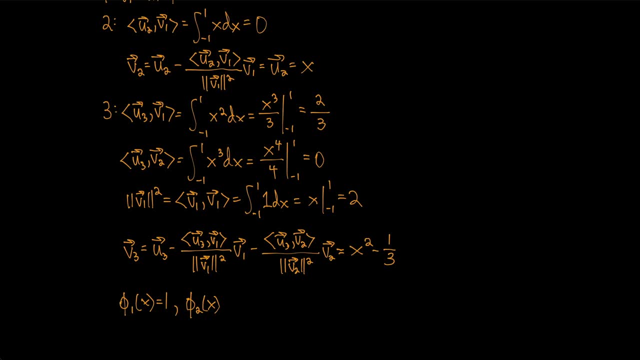 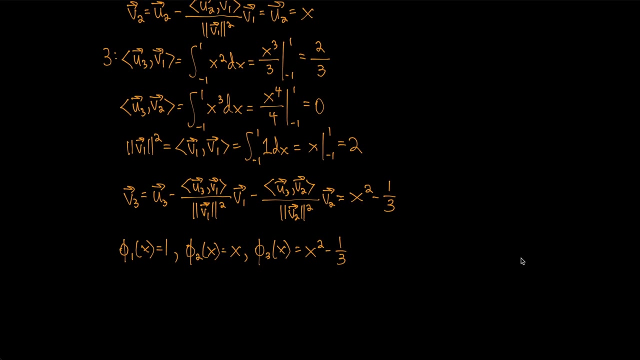 v2 of x is x as it was before, But v3 of x is x squared minus 1 third. So we had to subtract off a third in order to make these polynomials orthogonal to each other. These polynomials, by the way, are called the 1x and half 3x squared minus 1.. 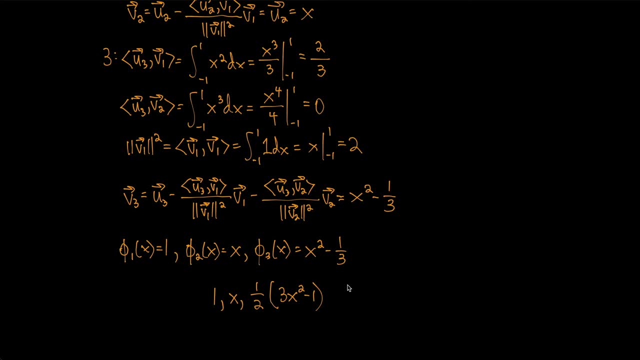 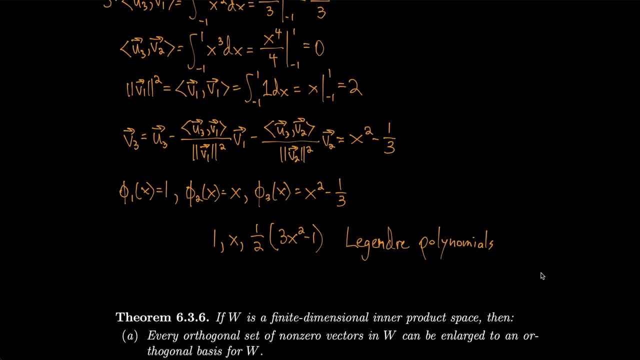 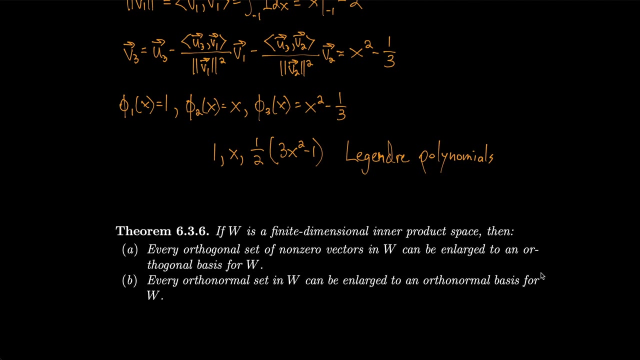 So if you just scale it a little bit, then these are the Legendre polynomials. They have a special name. If w is a finite-dimensional inner product space, then every orthogonal set of non-zero vectors in w can be enlarged to an orthogonal basis for w. 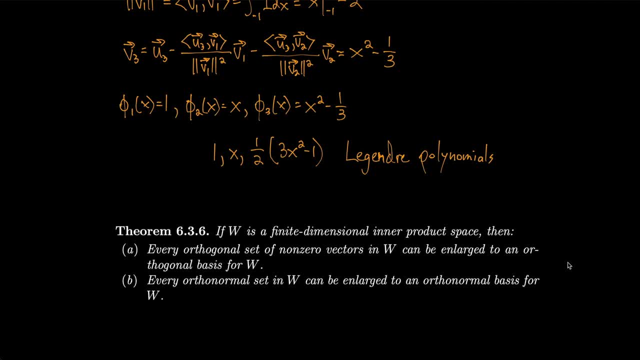 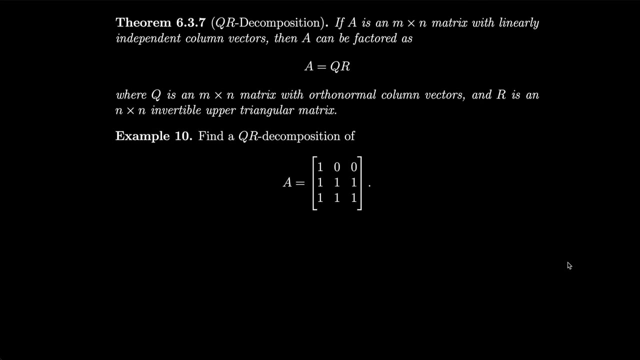 and every orthonormal set in w can be enlarged to an orthonormal basis for w, kind of like the way that we used to enlarge linearly independent sets into bases. Thanks for watching. If a is an n-by-n matrix with linearly independent column vectors, 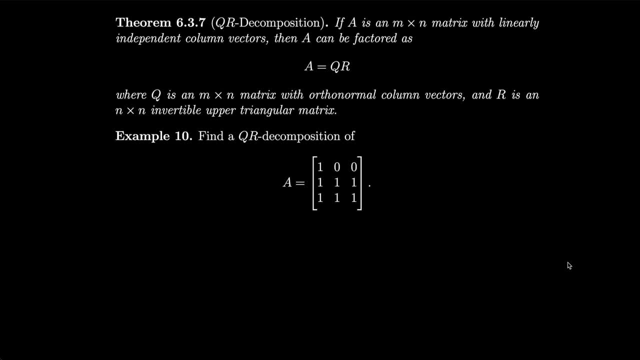 then a can be factored as a equals qr, where q is an n-by-n matrix with orthonormal column vectors and r is an n-by-n invertible upper triangular matrix. This is called qr decomposition. So how about we find a qr decomposition of this matrix given? 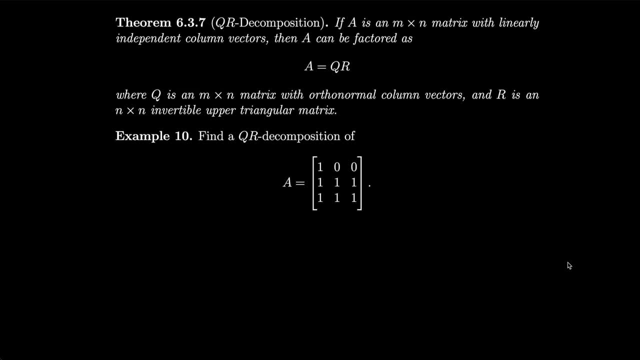 So what we can do is we can write each of the columns as as their own vectors. u1 can be 1, 1, 1.. u2 would be 0, 1, 1. And u3 would be 0, 0, 1.. 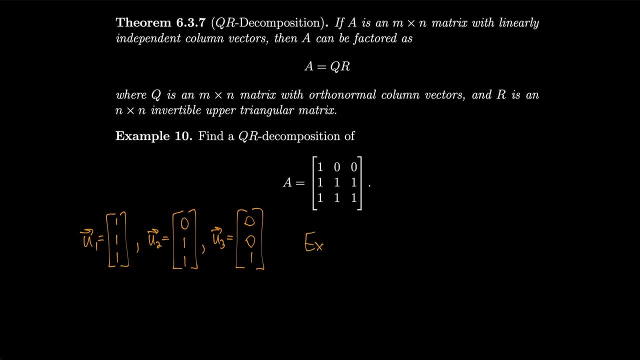 So then, by example 8, we have that q1 is equal to 1 over square root of 3, 1 over square root of 3, 1 over square root of 3.. Because, if you haven't noticed by now, 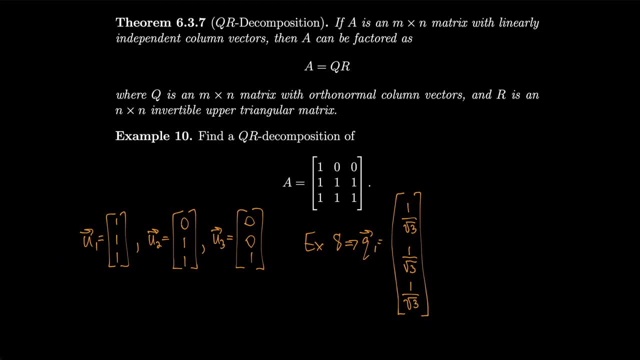 these are literally the vectors that we found an orthonormal basis for in example 8.. Otherwise, this would be a lot of work right now to try to figure out how to do it. So let's try to find the orthonormal column vectors. 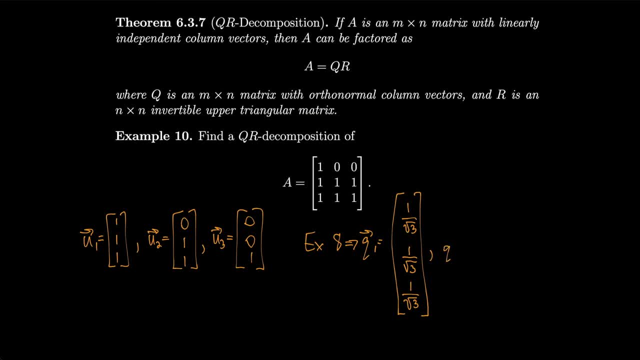 because we'd have to use Gram-Schmidt again. q2 from example 8 was negative, 2 over the square root of 6,, 1 over the square root of 6,, 1 over square root of 6.. And we had q3,. 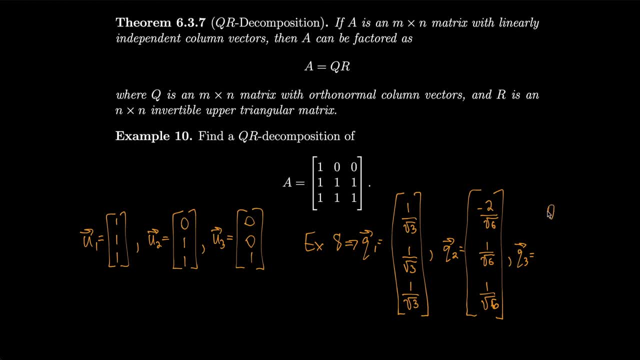 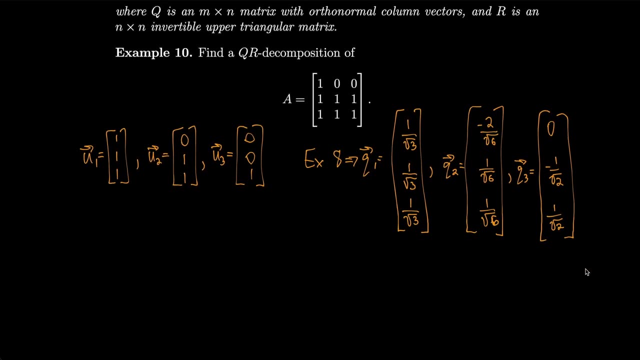 calculated to be 0, minus 1 over rad 2, 1 over rad 2.. Okay, so now we can write r. The matrix r will be given by it's an invertible upper triangular matrix. it's going to be given by each of the inner products of u with the column vectors. 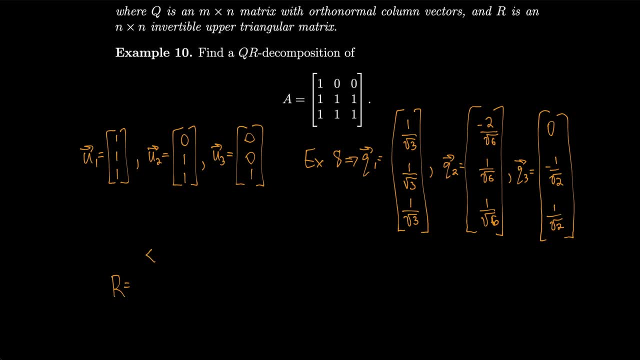 So the top left will be inner product of u with q1. And then we'll have or u1 with q1. And then we'll have our next entry, u2 with q1. And u3. And u3 with q1.. 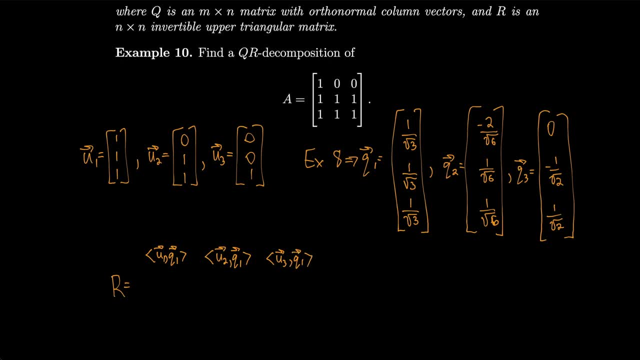 And then its upper triangular. so we'll have zeros over here And we'll fill in the rest of entries u2 with q2, u3 with q2, and u3 with q3.. And that's how we build a matrix. 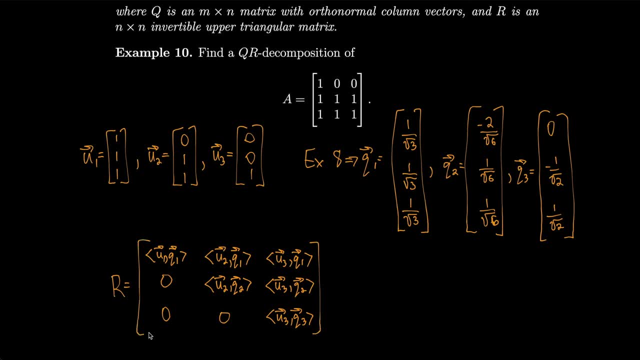 And then we'll have our next entry, u2 with q1.. And that's how we build the matrix r Computing each of these internet products. we get 3 over rad 3,, 2 over rad 3,, 1 over rad 3,. 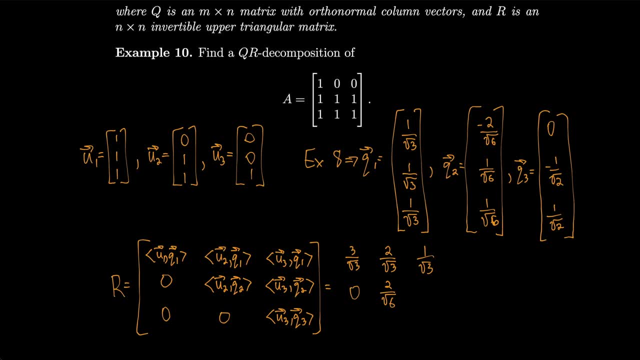 2 over rad 6, 1 over rad 6, per my zeros, and 1 over rad 2.. I'll load the first thing I mean before I run the second test. So we'll write forward here and it will change back to v as n mama, because we are saying: